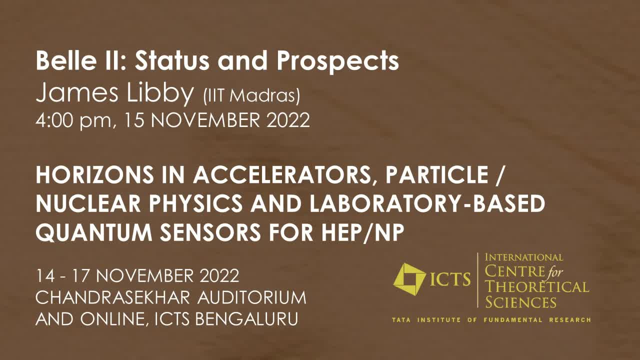 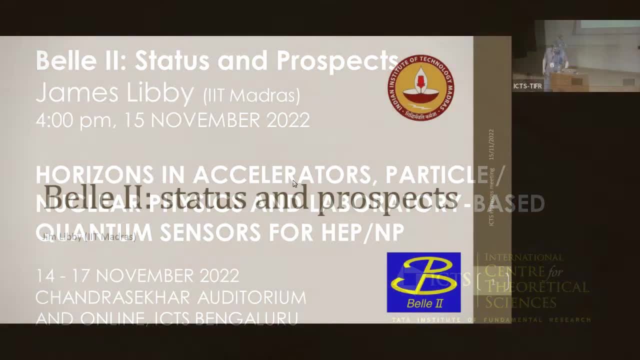 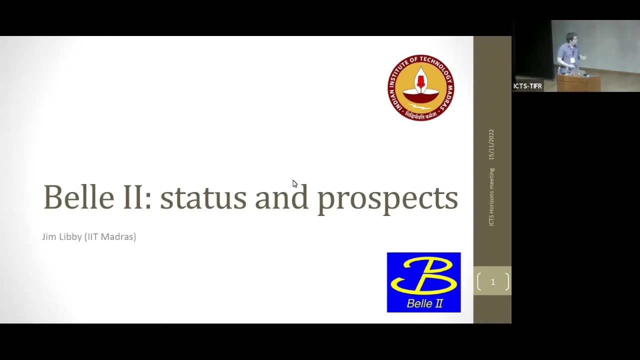 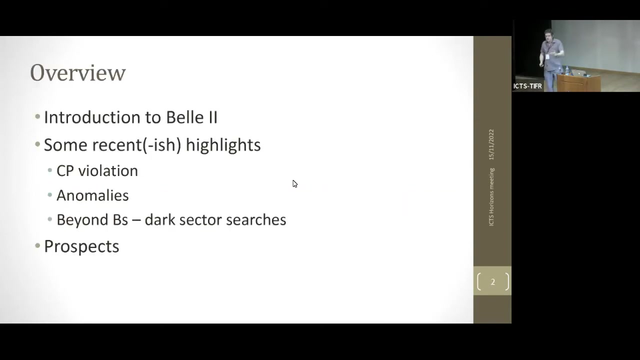 Okay. so thank you, Sudhir, and thank you to the organizers for inviting me to give this talk. So, as stated, I'll be talking about Bell 2 and its prospects. So initially I'll just introduce Bell 2.. This is the only talk on flavor physics here at the meeting. 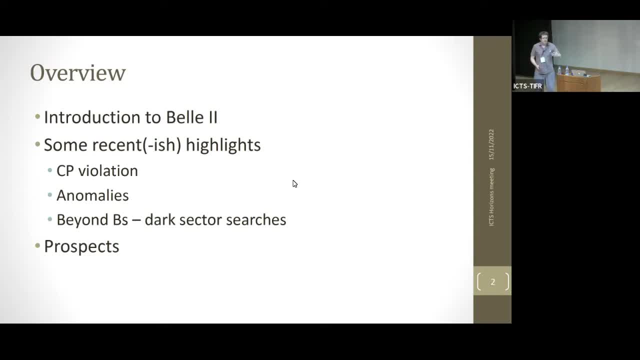 So that'll be quite a lengthy introduction. Then I'll talk about a few recent highlights. We're running an experiment, We're producing results, So I'll give just three examples: one related to CP violation, one related to the anomalies that Rukmini talked about just before. 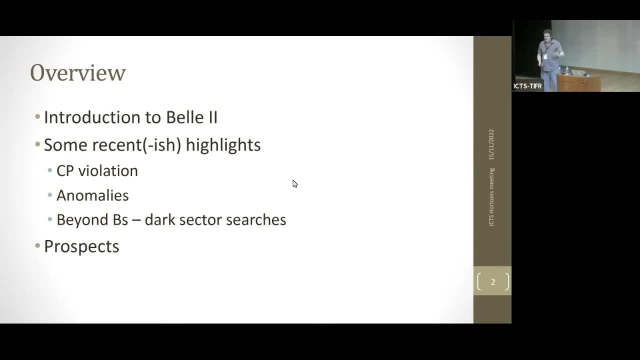 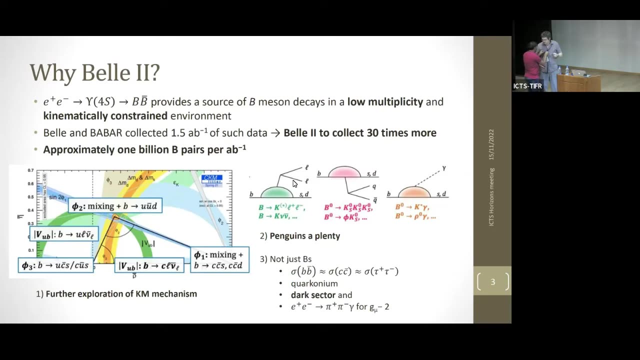 the tea break and then also explain- we're not just about B physics. I'll show one measurement that comes from a search in the dark sector before I conclude, talking about prospects. So why Bell 2?? So hopefully that's better, That's static. So Bell 2 is an experiment that predominantly 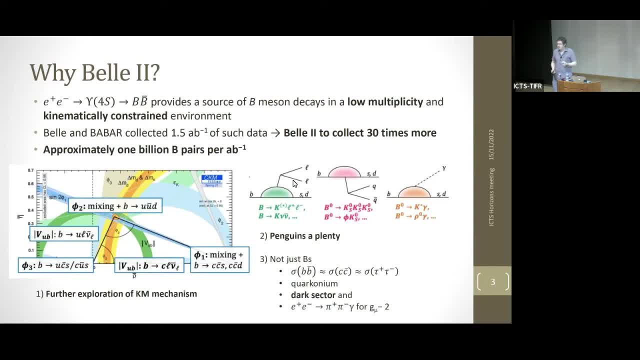 runs at the center of mass energy, of the epsilon 4s in E plus E minus collisions, and produces BB bar pairs. So we're a B physics experiment primarily, And this environment is just above the threshold for production, just over 10 GeV in center of mass. 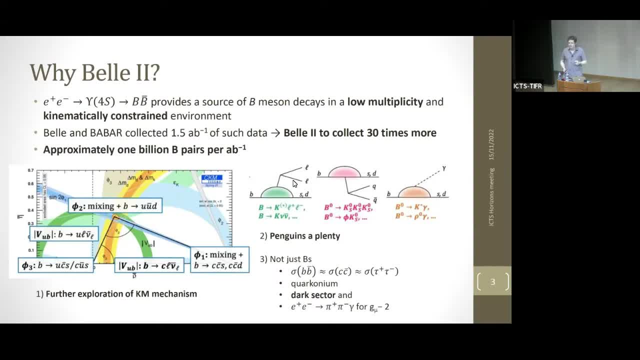 So the Bs are produced in a low multiplicity environment. There are no accompanying particles apart from the B mesons, And also, being E plus, E minus, we have very good kinematic constraints. So it's also built on a legacy and I'll talk more about that in a moment. 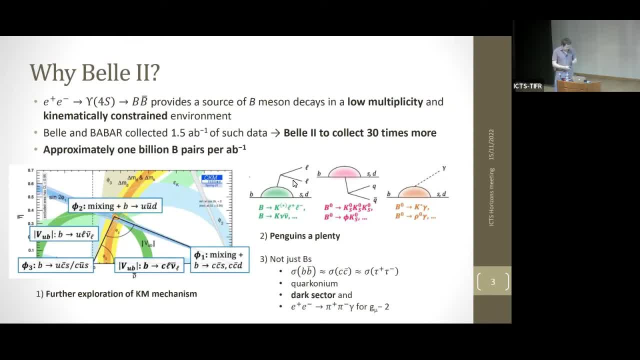 But there were two predecessors, Bell and Bell 2, not Bell and Bell 2, Bell and Babar, which collected one and a half interdefs at a bonds of data, And the goal of Bell 2 is essentially to expand that data set by a factor of 30. 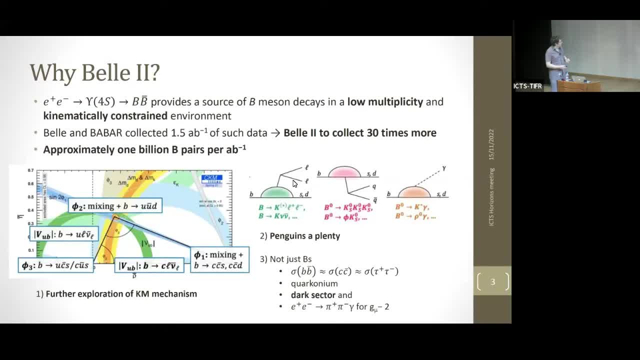 to get up towards 50 inverse Atobans. So just to set the scale, because I'll compare it to LHCb in a bit, one inverse Atoban is around 1 billion BB bar pairs. So there are three main goals. 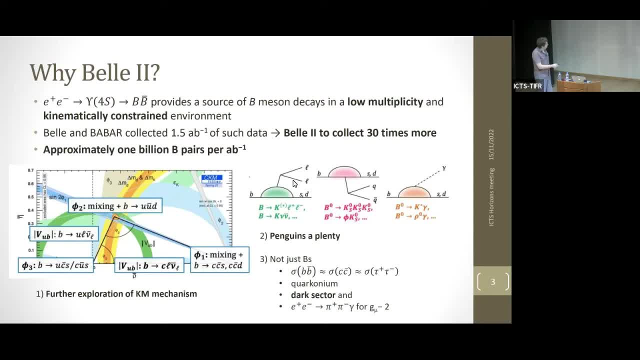 I would say in the Bell 2 program, The one we're famous for is the CKM metrology. This is measuring both the angles and the sides of the unitarity triangle, which I'll come back to, whether it be through semileptonic decays, through mixing or through CP violation. So the goal is to make 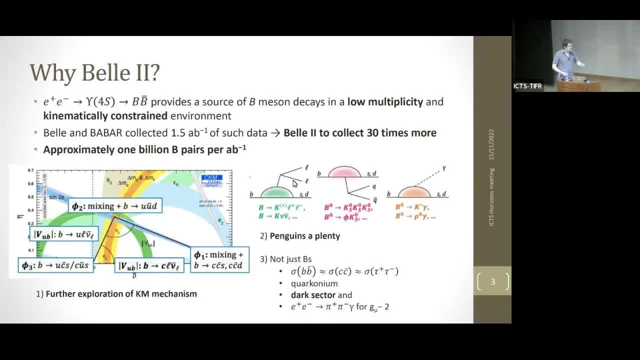 many such measurements and find some that disagree. some are more or less sensitive to new physics And in particular the new physics can enter in these flavor-changing neutral current diagrams. So we have many penguin diagrams of different types. We have so-called electro-weak 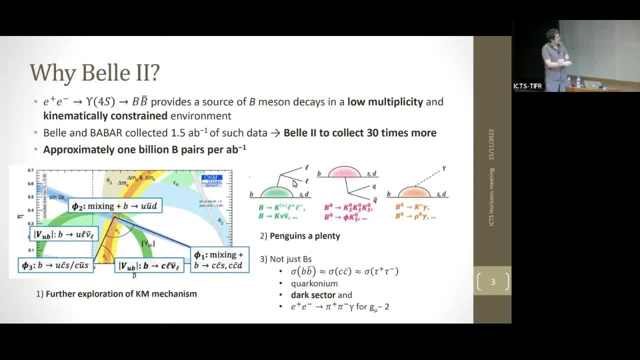 ones which lead to this B to SLL process. Then we have gluonic penguins, which give a hadronic final state but also potentially contain new physics within this loop, And then we have the purely radiative penguins, which I won't have time to talk about, but that's a very important part of our program. 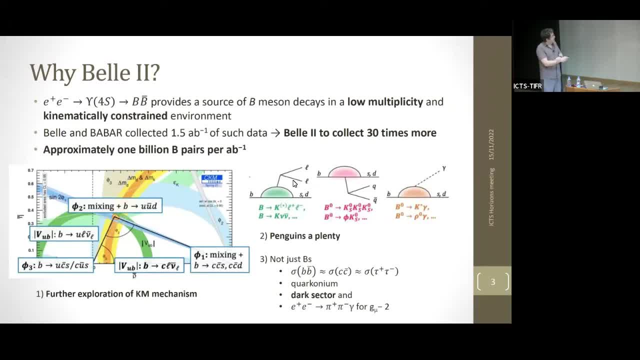 as well. But at this center of mass energy and E plus, E minus collisions, it's not just Bs. The cross-section for charm and for Tau's is almost equal to that of B mesons. So we have very large charm samples and a very large number, in fact world-leading number, of Tau decays, as 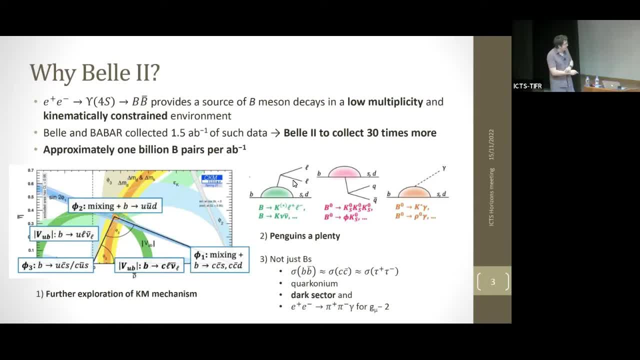 well. So we have very large charm samples and a very large number, in fact world-leading number, of Tau decays as well. There's also great interest in spectroscopy. that can be done both from B decays and also in ISR, where you reduce the center of mass to produce. 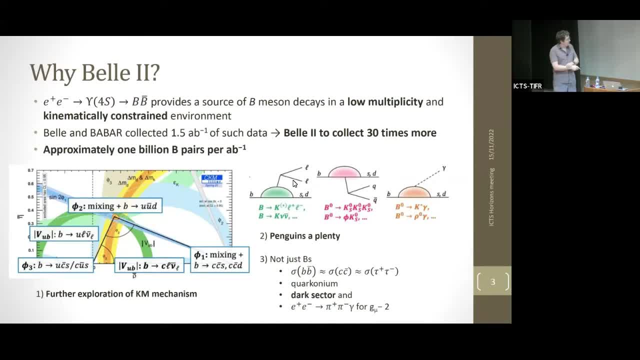 exotic states in the Charmonium region. I'll talk more about the dark sector. And then there's this important contribution of measuring low multiplicity. final state: E plus, E minus to pi pi gamma, which goes into the calculations of G minus 2.. 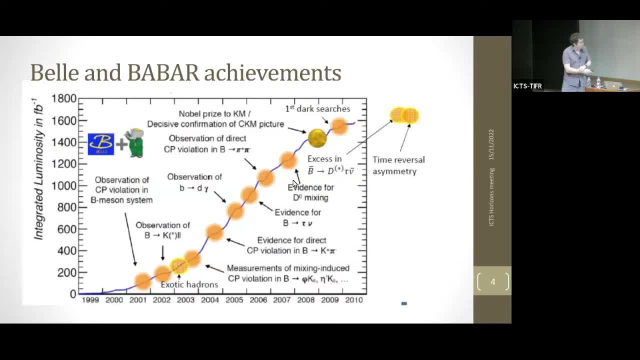 So, as I said, this is based on success from earlier experiments- Bell and Babar- So this is, as a function of running time, various measurements that were made by Babar and Bell over time- And they encompass rare decays. 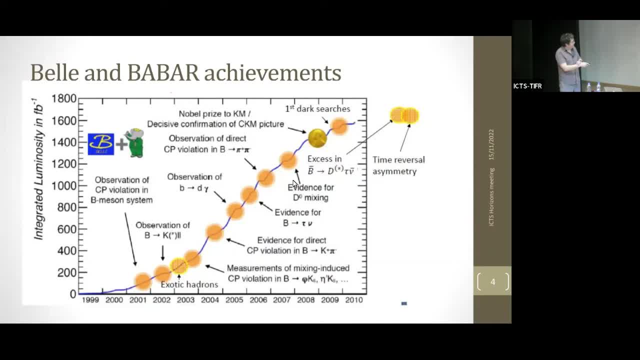 the first observation of beta-KLL, the first CP violation in the B sector which led to the Nobel Prize for Kobayashi and Muscawa. And then there's the beta-D star, the first D star, Tau measurements, the first of these various exotic hadrons, dark sector and other things going. 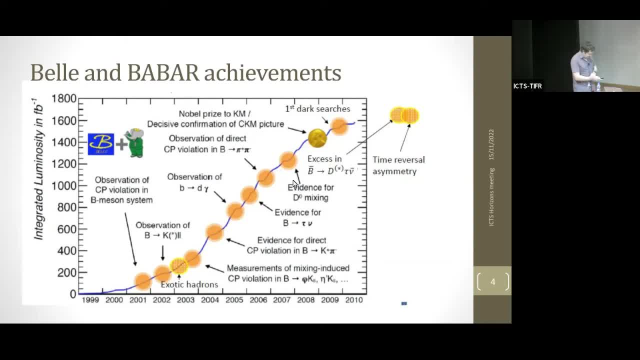 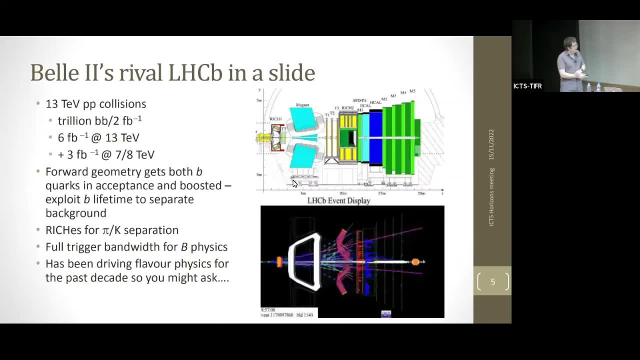 on, But you see, this program finished in 2010.. So in the last decade or so, flavor physics has moved elsewhere. And now the leader which I should talk about is LHCb, which has been running very successfully since the start of the LHC. They exploit the very large cross-section for 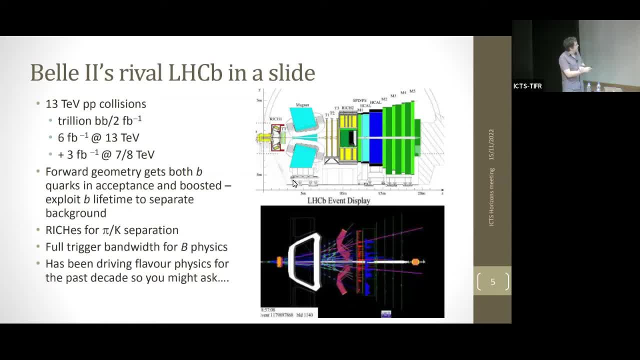 BB-bar production in proton-proton collisions at the LHC And this leads to trillions of BB-bar events per two inverse femtobytes. So they've collected nine inverse femtobytes of data so far. They're a dedicated experiment. 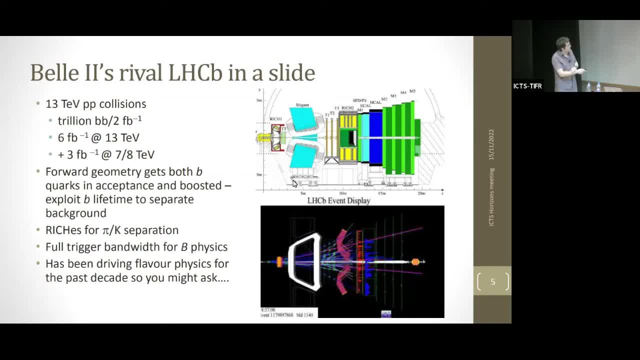 having a forward geometry, with the Bs boosted into the acceptance So they can exploit the displaced vertex. They've installed excellent particle identification detectors And they can also dedicate the whole of their trigger bandwidth to flavor physics. So, and now they're going to 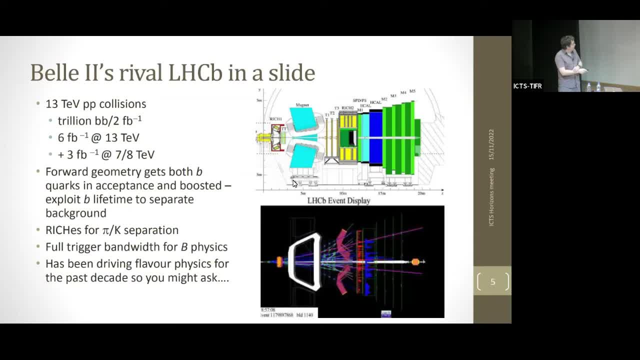 run with 40 megahertz readouts or have started to run. So they've made many measurements that Rukamini showed And they've also made many measurements that they've used in the experiment And also have made great impact on those unitarity triangle measurements. So but 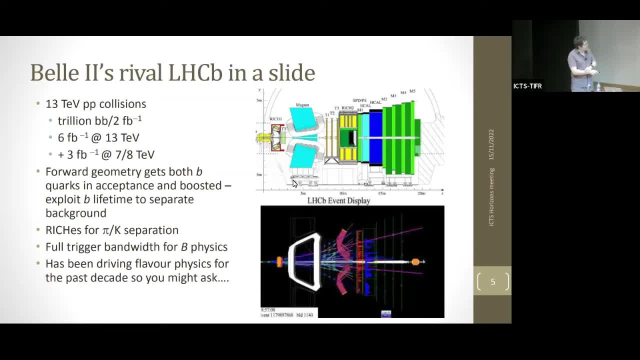 just to give you a sense. if you can see, in this event display picture there's a very busy environment. Here is a Bs to mu mu event or candidate. You see the two muons going through, but there are many, many other tracks And the events are not as clean as what one gets at an 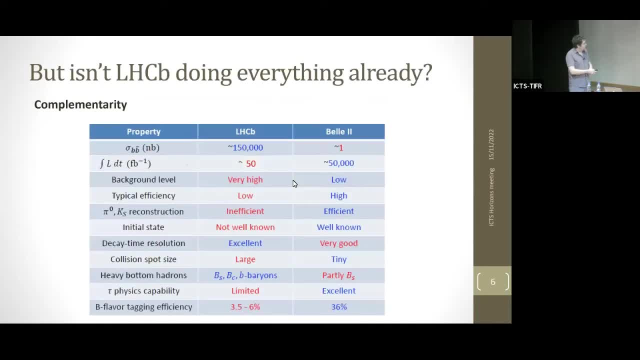 E plus, E minus experiment. But given its success, you might ask yourself why we're still doing flavor physics somewhere else, And the answer simply is that there is complementarity between the two programs. So, even though we suffer from having a much lower, 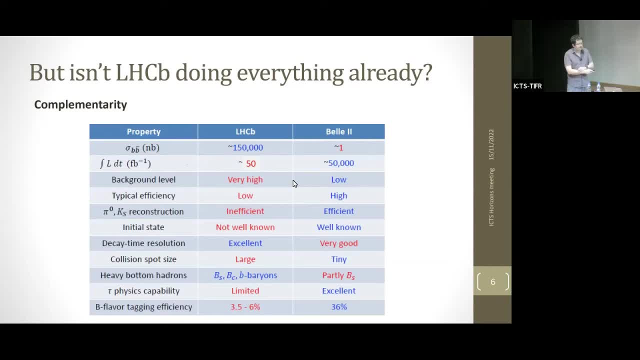 cross-section at bell two. we're trying to compensate for that by having a very large luminosity, And I'll talk about how we do that in a moment. We have lower backgrounds. We have higher efficiencies. We have almost 100% trigger for BB events. We can reconstruct neutral particles. 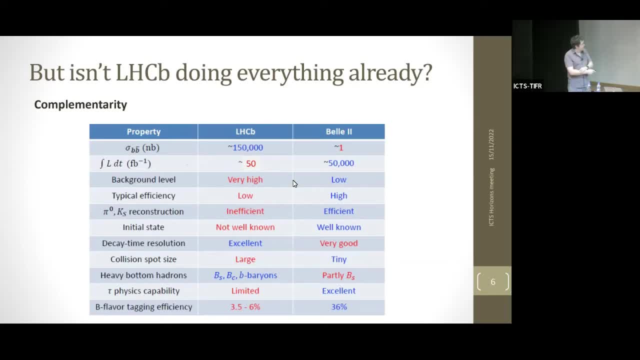 very well. We have well-constrained kinematics. We don't quite have as good decay time resolution because the boost is lower, but we manage. And we have a very tiny beam spot now which helps. We don't produce B mesons other than the. 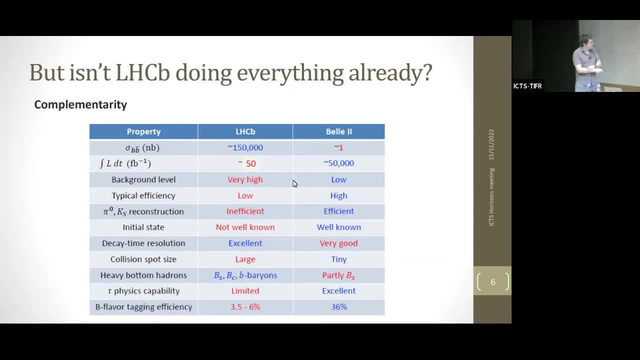 B plus and B zero. very much We could run at the 5s and produce Bs mesons. This was done by Bell. They has a sample of the Bs Bs bar produced there. We have this tau physics capability And we also do very well in CP violation measurements by boosting our flavor tagging efficiency. 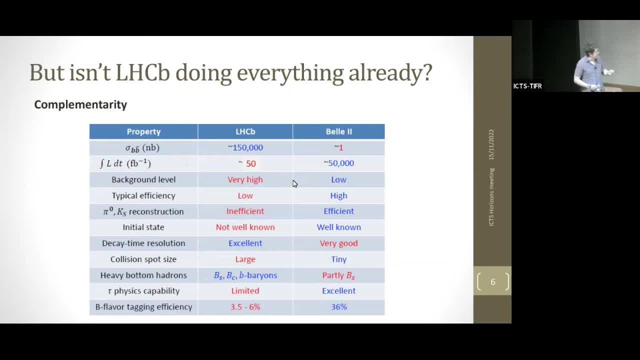 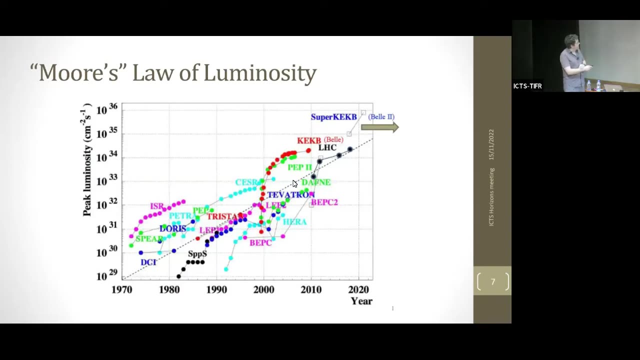 The B zero and B zero bar pair are produced in a quantum correlated state, which means that we get a much higher efficiency And we have a very tiny beam spot now, which helps. We don't produce B mesons very well. We run at 0.25 and B minus and takes 12ylum vertical. 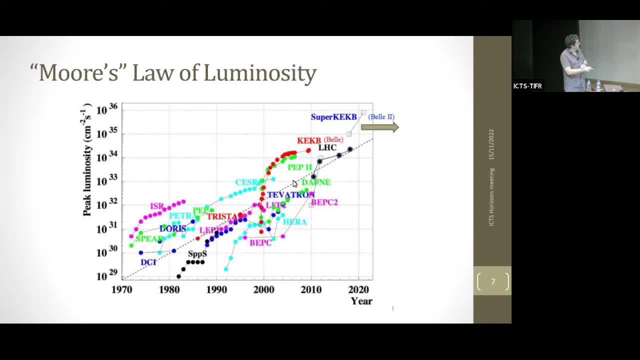 This accelerator for Bell was the world's leading in terms of instantaneous luminosity, And this is the projection for SuperKB. We haven't achieved this, so we've gone off the end of this chart, but we're closer to this line now which is going to try and push up that luminosity to well above 10, to the 35.. 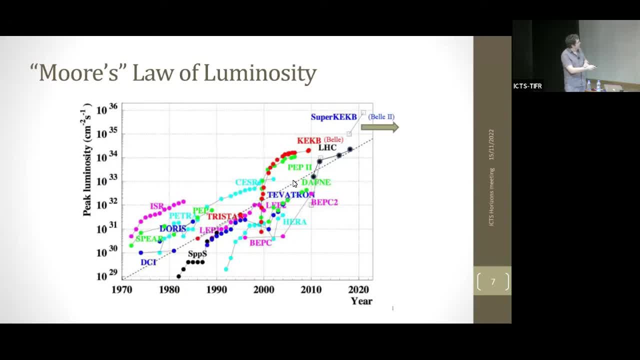 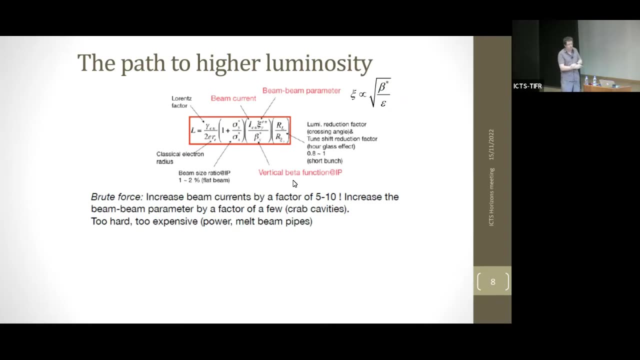 In fact, 6 times 10 to the 35 is the target, And currently we're running at 4 times 10 to the 34 is the record that we have reached so far. So how do we get this increase in luminosity? So in this formula here there are various factors on which the luminosity depends. 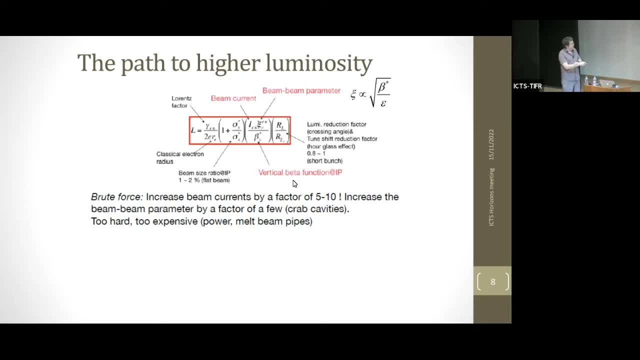 There are two most important parameters here, of course is the beam current, which you can increase to increase your luminosity, or you can decrease this beta star function, which is basically making the beam size in the vertical direction at the interaction point very, very small. 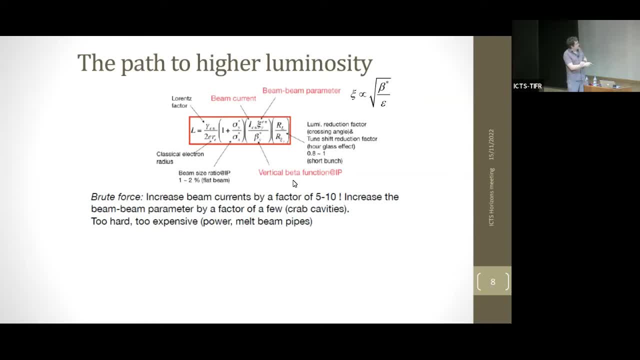 You have to pay attention to this beam-beam parameter as well, which is actually proportional. So if you make this beta star smaller, you also reduce this parameter, So you have to make sure that your emittance also decreases in a similar way, so that this doesn't destroy the luminosity gain you're getting from the increase in beta star. 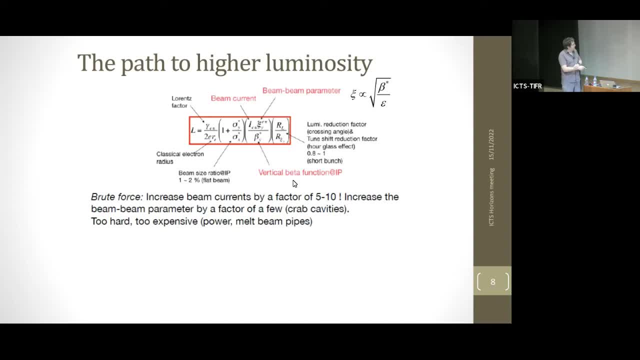 So there were brute force ideas. You just increase the current, but that doesn't really work so well. It's very expensive because of the RF costs and it would also create so much synchrotron radiation. it's very hard to make the beam pipe. 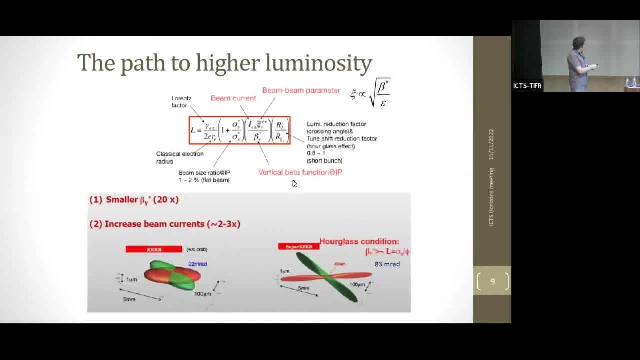 So another solution was just So. another solution was just to make this beta star 20 times smaller than Super Keck B. And these cartoons here show the bunches crossing. This is what happened at Bell. There are these sort of Gaussian-like ovals of positrons and electrons crossing. 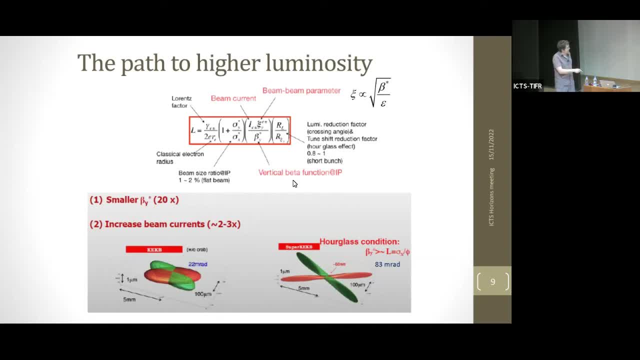 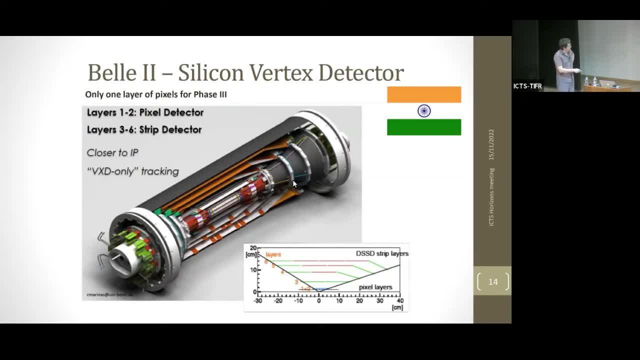 But at Bell 2 and Super Keck B, due to a very elaborate final focus, which again was talked about by Frank yesterday, we can get a very small crossing region due to this hourglass shape of the bunches, the readout, there's this, uh, so there's this chip on sensor design, so called origami, to keep, 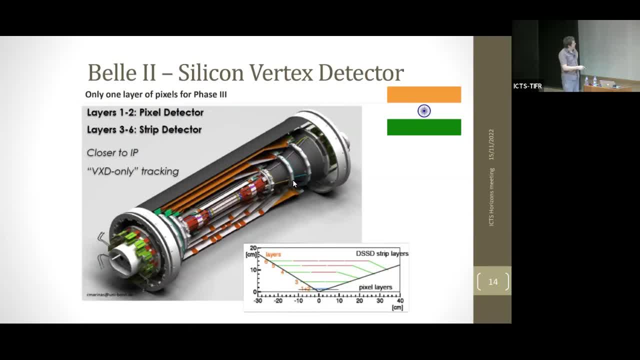 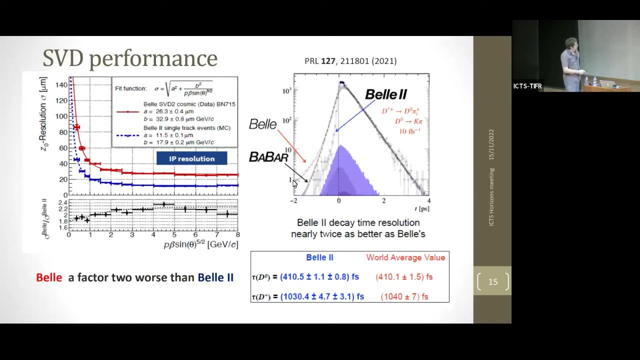 the readout close to the sensors and the mass low, and we were a key part of this, and various contributors from other institutes, as well as the leadership from tifr. we we've successfully contributed to this detector working. and to prove that it's working, a couple of plots and one. 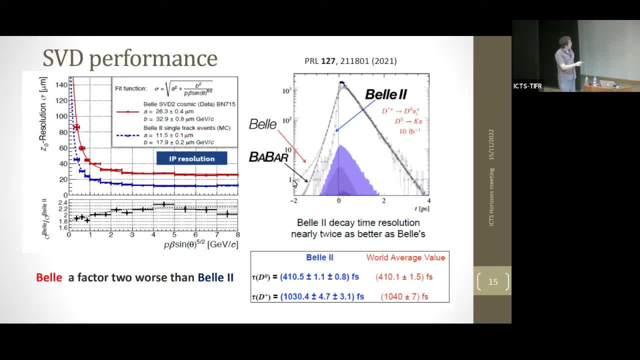 publication here. so, um, this is the impact parameter resolution as a function of a variable that pretty much depends on the momentum, taking into account the angle at which the particle traverses. the silicon and the red is the bell impact parameter resolution and the blue is what we now have in bell two. this is, this is a, a, a, a prediction. this isn't actually the data, but we've 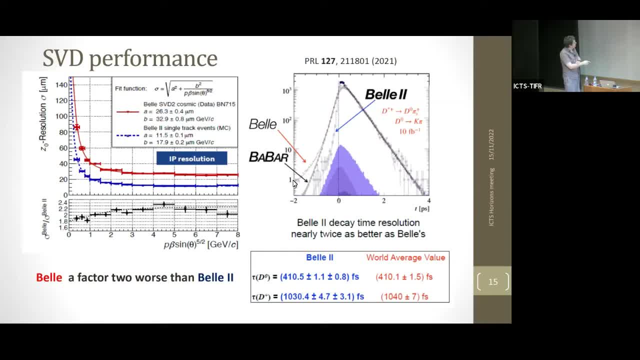 matched up to this when we we actually looked at this. i should have replaced this plot in fact, and as you can see, it's almost a factor of two- improvement over the former full momentum range, so that leads to physics and one of our early publications. we actually now have three such. 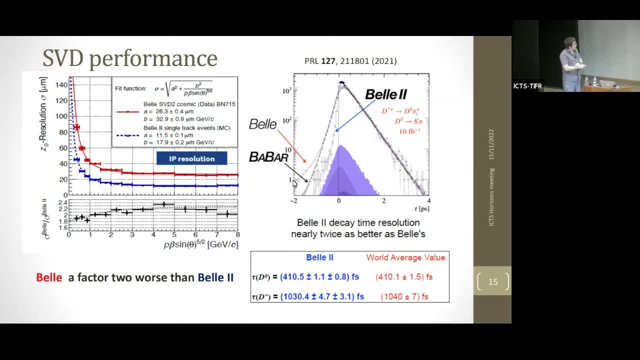 publications are measuring charm lifetimes. so here is the distribution of the charm lifetime measured in the detector for d0 decays which are tagged coming from a d star that cleans up the sample. this is d0 to k, pi. and on on this side, uh, you, you, you can see that, the charm. but on the negative side, you're seeing the resolution. 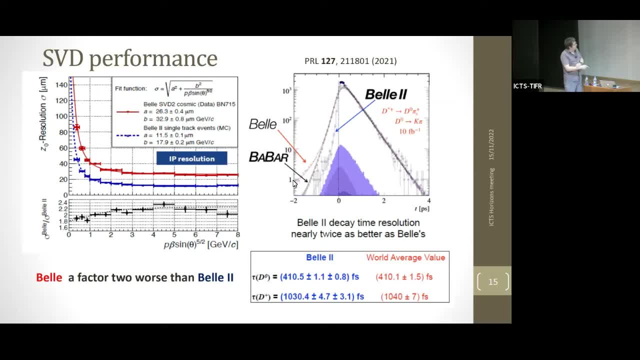 that you have on the lifetime and, uh again, the. this, this plot here, shows the improvement that we get from bell two. this is this line here and this was what baba and bell had. so there's a significant improvement and this has been leveraged to get world-leading measurements of the d. 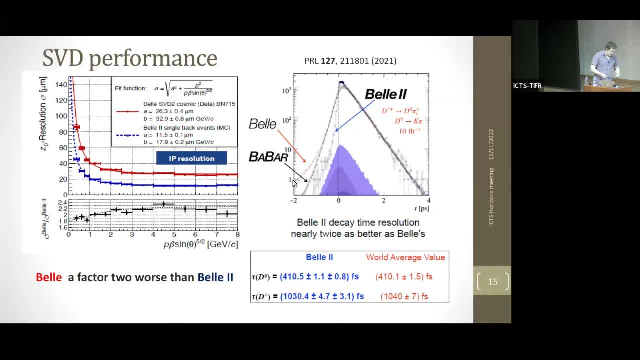 lifetimes, which are important in terms of qcd predictions for these and also as benchmarks for other lifetimes in the charm sector. so that's, uh, an introduction to the detector, and i want to talk about various parts of the physics. so the first of these is just a little bit about cp. 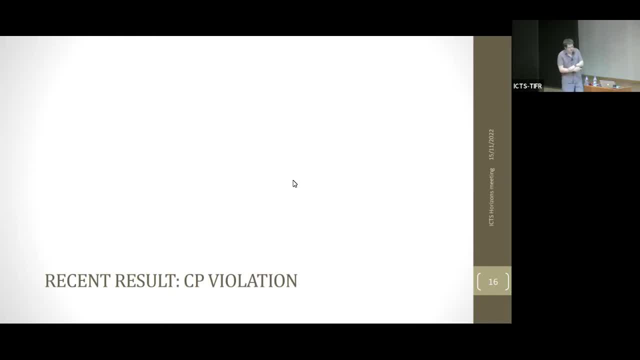 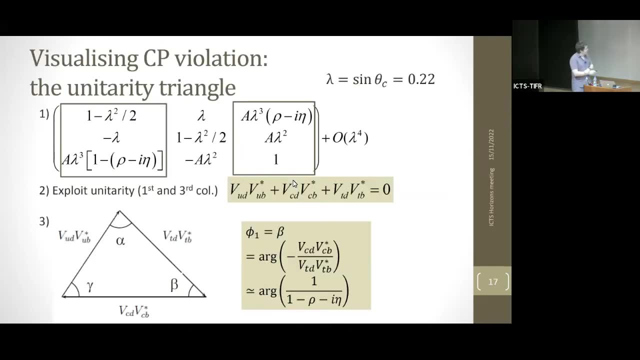 violation and showing that we're prepared now to make, uh, accurate measurements of interesting processes in in cp violation, and to do that first of all, i just want to say a bit more about the ckn matrix, which was shown to you by rukmini in the talk before the tea break that we we like to use. 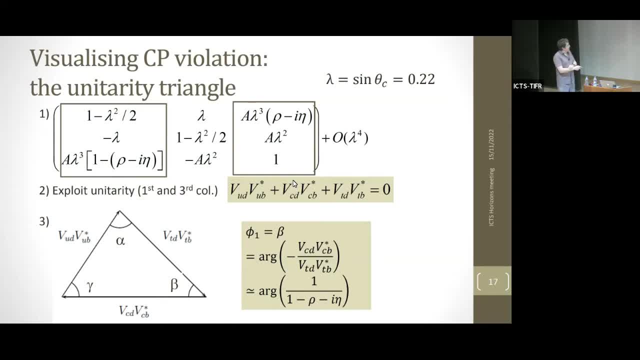 this wolfenstein parameterization, where this lambda parameter is an expansion parameter, that is, the the sign of the kabiba angle, which is around 0.22. so we we first of all write down the terms up to third order in this lambda parameter, and what you see by this is that the 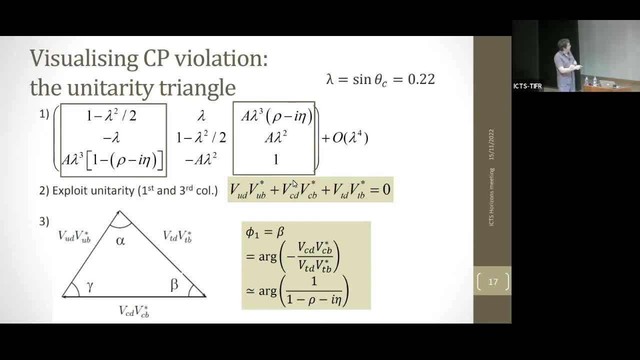 these other parameters, this a rho and eta are there and they tend to sit in these uh terms which which are coupling together the first and the third generation. And, importantly, eta is the one that makes these elements complex, And the complex nature of these elements is what ultimately leads to the CP violation. 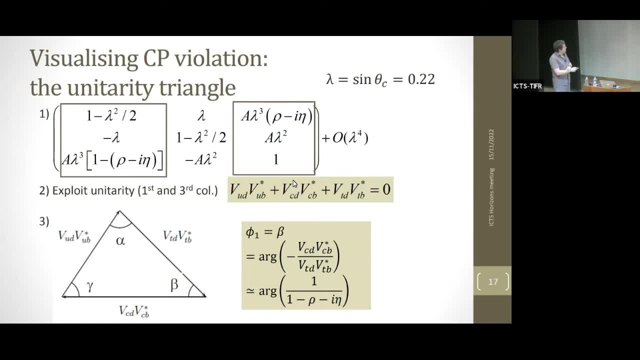 So we exploit this relationship to combine together the first and the third column And that can be seen as just adding together three complex numbers And they have to sum to zero. So that gives us a unitarity triangle. But what's nice about the first and the third column? 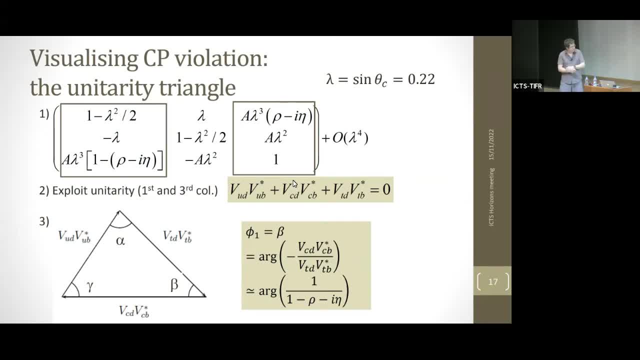 is that all of these terms are of the same order. in lambda They're all lambda cubed. So the lengths of the sides are approximately the same length. So in the B system each of these sides depends on some coupling of the B. 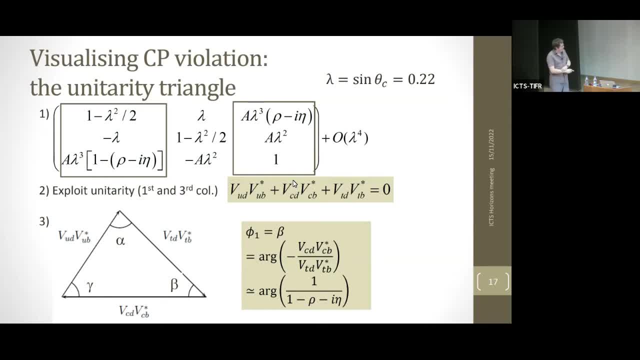 either to the up quark, the top quark or the charm quark. So using B physics allows us to measure everything and more about the unitarity triangle And the key measurement that was made that showed that the Kobayashi-Maskawa mechanism. 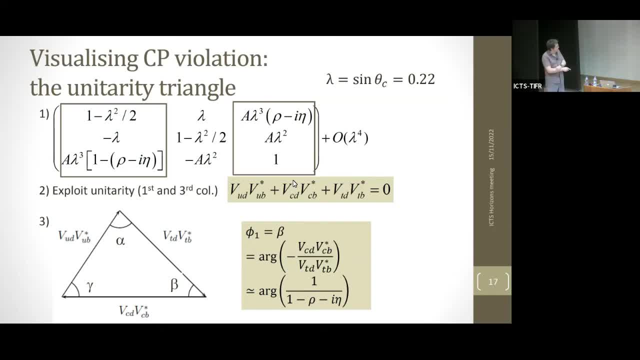 was correct in describing CP violation in the standard model was to measure this angle beta down here which can be cleanly represented, And this is related of course to this eta parameter And this is sine 2. beta measurements were key to the initial B physics program at the B factories. 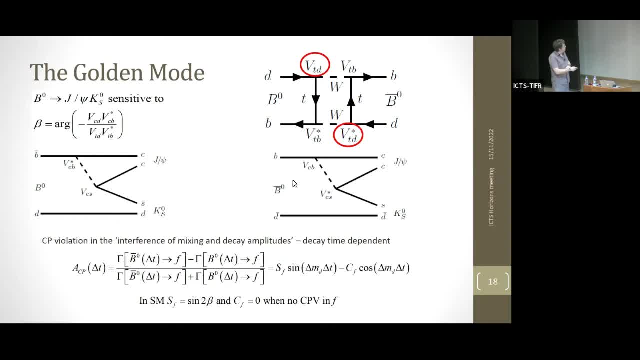 So how this measurement works is that you take a final state of the B decay to CP eigenstate, in this case J psi K short, And this final state can be reached in an identical fashion for B zero or B zero bar. However, because the B zero and the B zero bar mix, 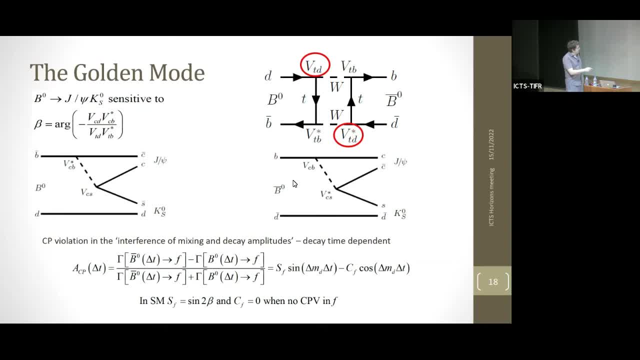 you don't know whether it decays before or after it's mixed And therefore interference builds up And that interference, because of this box diagram, depends on DTD which, if you remember from the previous slide, is one of those that depends on eta, and it is complex. 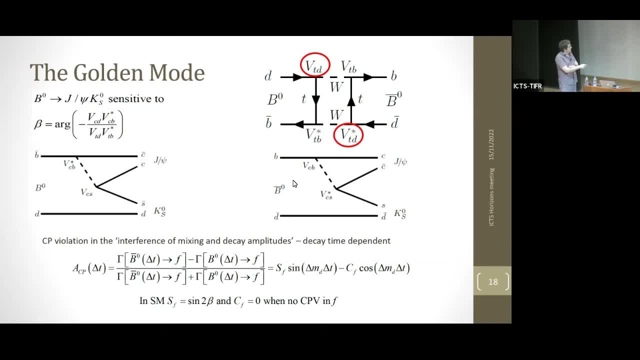 So you can measure the CP violation by measuring how this varies as a function of time. because you can measure the CP violation by measuring how this varies as a function of time. because you can measure the CP violation by measuring how this varies as a function of time. 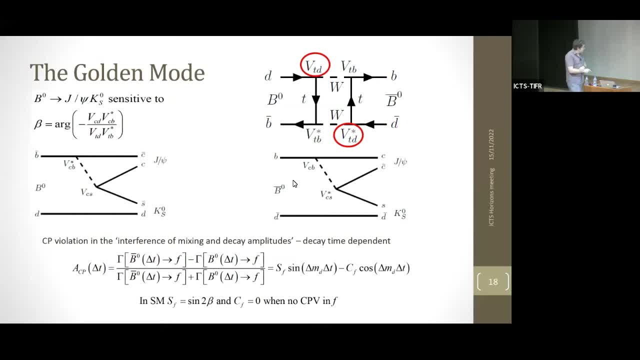 depending upon the oscillation. So you build up a time-dependent asymmetry which depends on the difference in time between the two decays. I'll explain that on the next slide. So you just look to see how many B zero bars were born, decay to this final state. 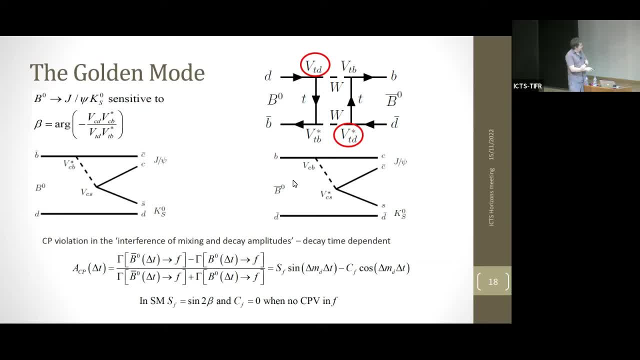 and B zero as a function of time. And you work this through and you find that the coefficients of the two terms that depend on the mixing rate. for B, mesons, delta, MD, there's a sine term where the coefficient is exactly sine 2 beta. 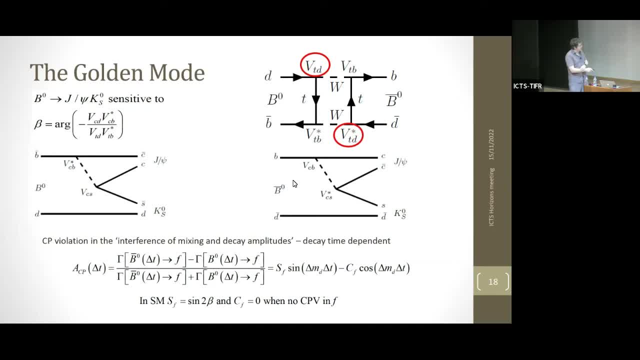 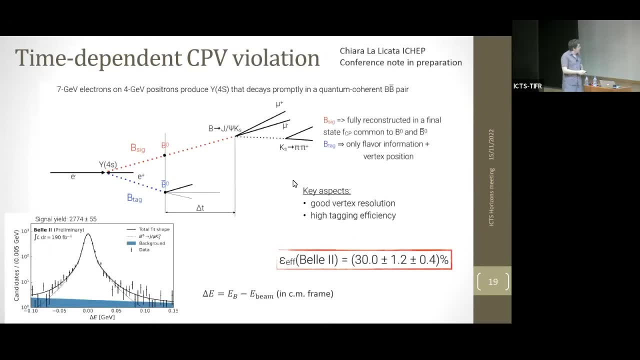 and you have a cosine term which would lead to direct C, and you have a sine term which would lead to direct C and you have a sine term which would lead to direct C, which is actually zero in the standard model. So we made our first measurement of sine 2 beta at Bell 2,. 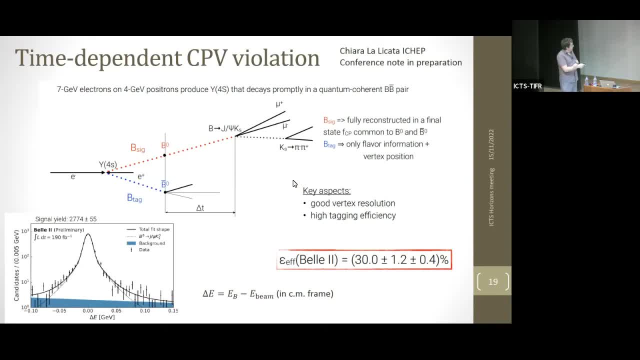 and presented it at iChat this year. So this asymmetry of the collider comes into play here, where our two Bs are boosted forward in the lab frame and they fly a significant distance before they decay And we rely on knowing the flavor of the B zero here in. 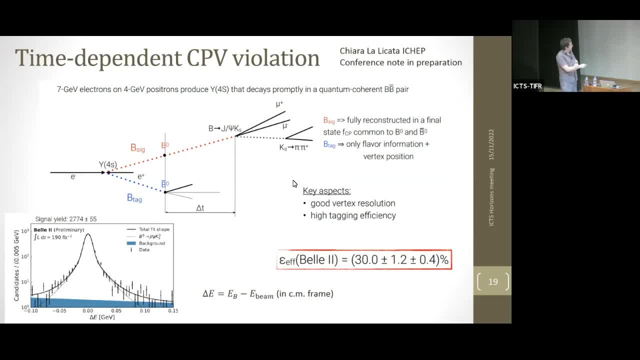 in red, that decays to our signal from the B zero bar on the other side as it decays. So if it decays to say, a lepton, we'll be able to tell what it was at this time And because of the quantum coherence. 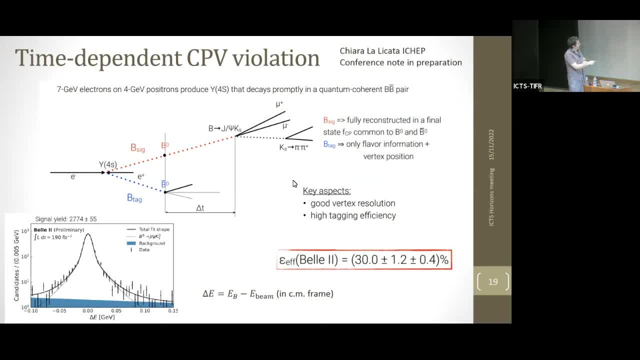 they evolve together until the point of one of them decays. And then we measure, as a function of the distance between these two decay points, how many B zero and B zero bars we see, And then this decays to a very clean final state. 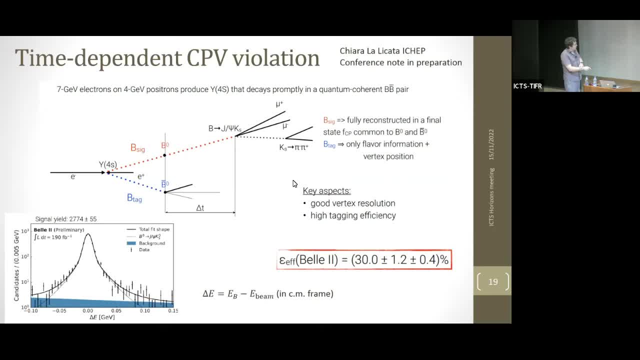 It relies on this tagging efficiency that we have- and this has been measured now to be around 30%, as expected- And it comes from the fact that this, this quantum coherence, means that we're not oscillating freely like they are at LHCb. 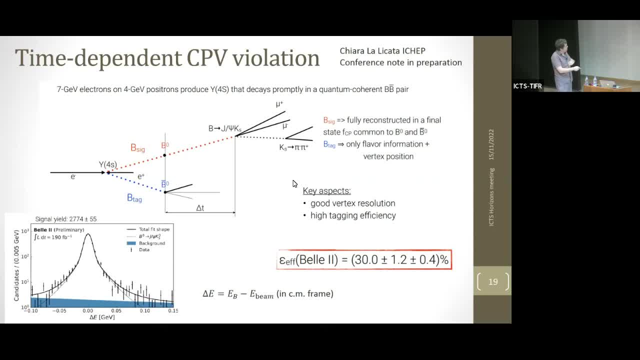 or even it can hadronize to something which you don't get the tag correctly and you rely on same side tagging and things which are much more difficult in a hadronic environment. So also we exploit our kinematics. This is one of our common variables: delta E. 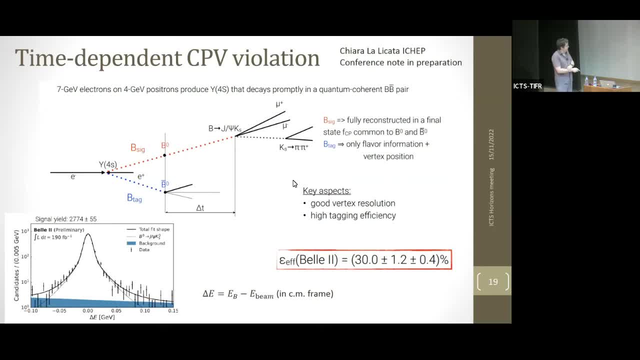 where the energy of the B less the mass of one of the beans in the center of mass, which is the energy of the B less than the mass of one of the beans in the center of mass- should be equal to zero. So we get a large peak of the signal here at zero in this J psi k short final state. 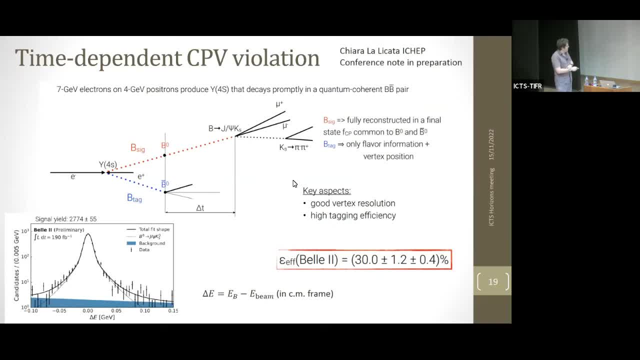 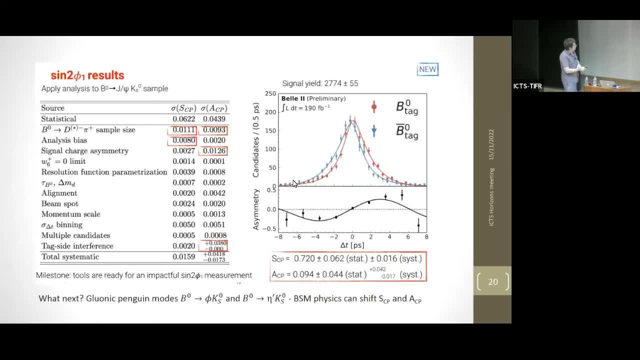 and we have nearly 3,000 candidates in the sample used for this analysis, with very small background. So those events are then taken and they're turned into a CP asymmetry. So the red are those who are tagged at the time of the first decay to be B zero and those B zero bar. 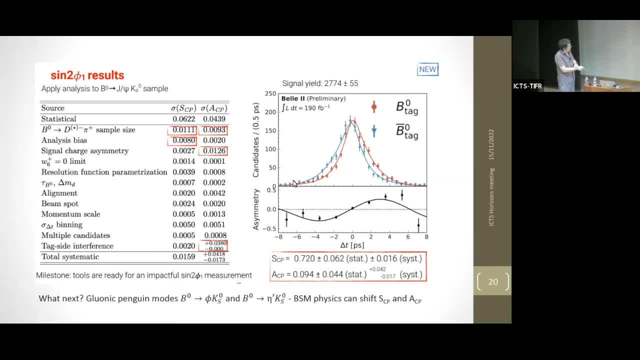 And you can see um. but if the, if the signal one decays first, you end up with a negative time difference and positive if it's um, it decays after the tagging one. but what you see is a distinct difference as a function of time. then you fit this nice sinusoidal form to it and you get out your. 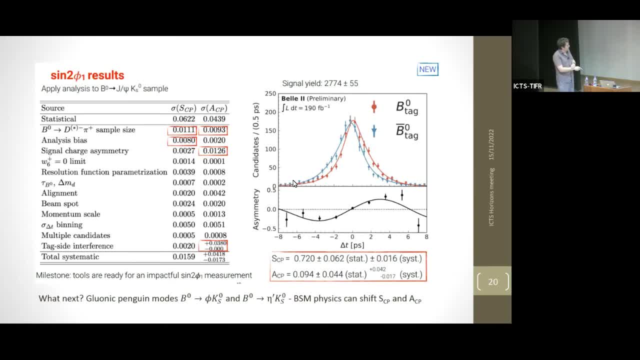 coefficient for the sinusoidal term, which should be sine 2 beta, and it agrees well with previous measurements and we don't see any evidence yet for any direct cp violation, also agreeing with the standard model. so this table of systematics i just flash here i think i shouldn't go into too. 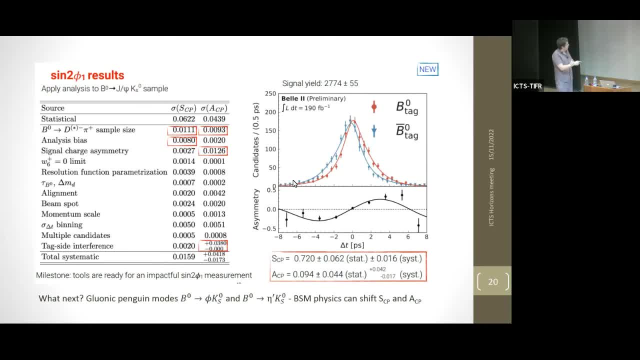 much detail given the amount of time i have, but it's important to note that many of these systematics actually will decrease with more data, largely data driven. there are things that we can understand better with more data, so why we're doing this, of course, is a validation to show. 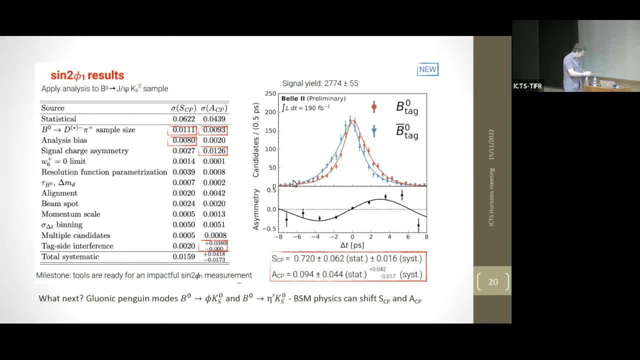 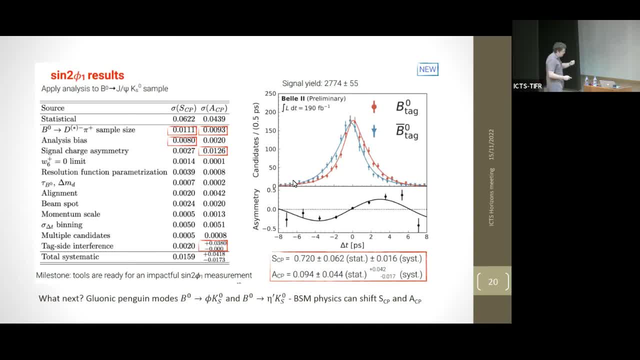 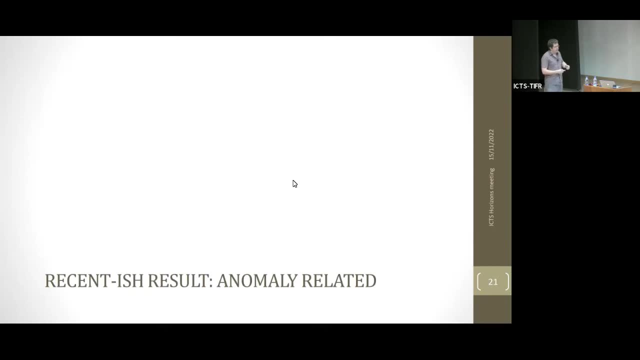 and a to prime k short where that gluonic penguin can play a role and potentially there's a new phase will come in which will shift the value of sine 2 beta. and those are the next measurements that we can expect now. we've done this validation using j psi k short, so moving on now to something. 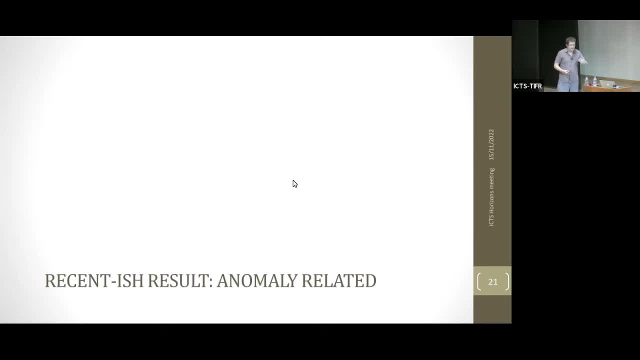 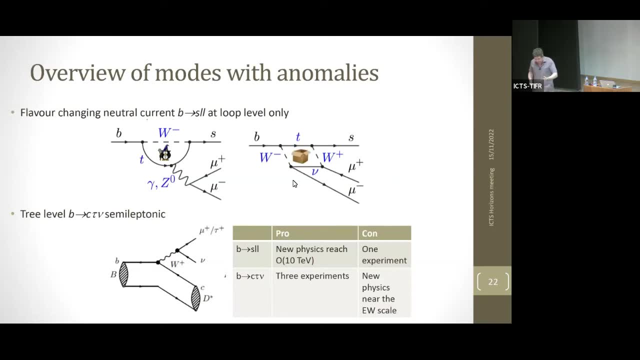 slightly more exciting. maybe we'll talk about a measurement that's related to the anomalies that were talked about. of course, ultimately we will look at b to s, l, l and also at b to d, star town u, and this is going to come probably relatively soon. however, we suffer statistically in this mode compared with lhcb. 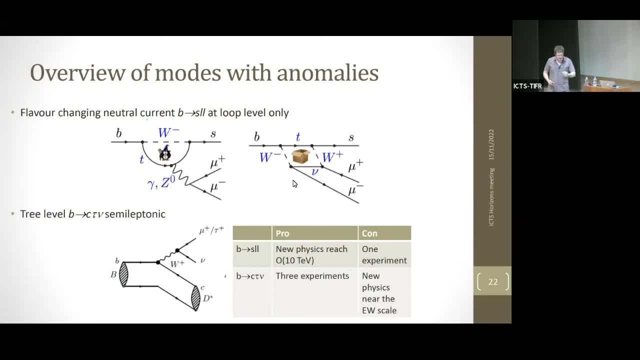 though we have a great advantage in terms of lepton universality that the efficiency for detecting electrons is almost the same as that for muons, which is very different to what happens in the general purpose detectors at the lhc. of course, as rookmini said, i should. 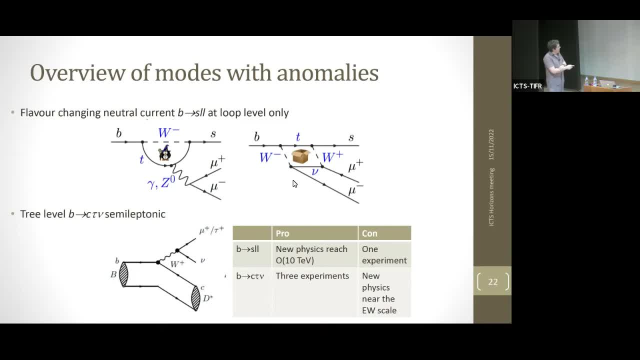 just emphasize. these anomalies are of rather different types: the flavor changing neutral current ones are completely dominated by loop processes. so there are many possible new physics explanations here. that's what's going on inside these loops that could change what we expect from the standard model. so that's the pro of these types of decays. there are many possible new physics answers to. 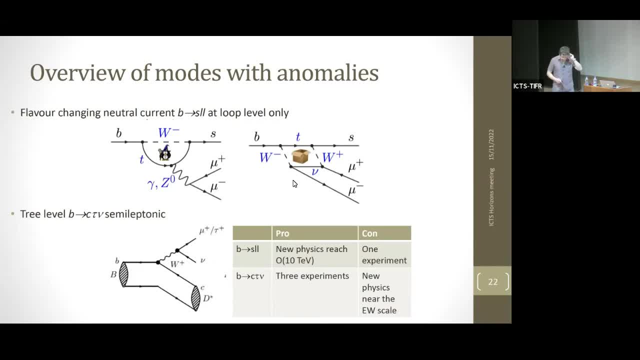 why they might differ. the con, of course, is there's only been observed by one experiment and ultimately, of course, we should make measurements that will, uh, see this, but we need many atoms of data to do so. for b to c, tau nu, this is is, you know, three experiments have seen the same thing, but it's a very hard measurement to make. 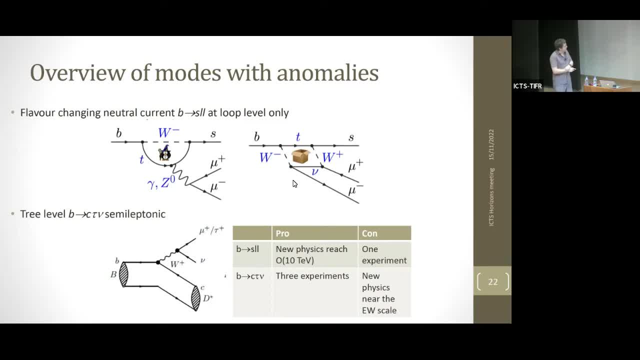 The backgrounds are very, very large, but they are different in the hadronic and the E plus, E minus environment. So we just need to measure this more precisely. But of course the physics has to be near the electroweak scale, because it's at the tree level in the decay that has 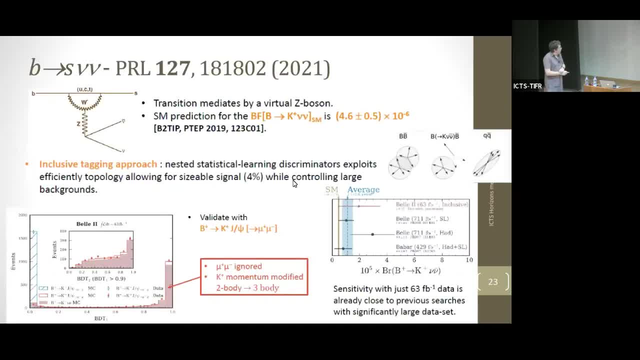 significant impact. So I'm not talking about to charge leptons, but there's something that's rather unique about the E plus, E minus environment that you can actually measure nothing very well. So we're looking at BS to new new bar. So this is one of these loop diagrams here where you just 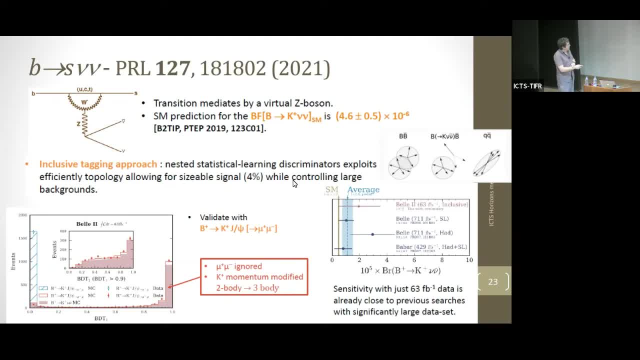 have a Z coupling to new new bar And this can be predicted reasonably well within the standard model, And this is obviously complementary to anything that's going on in the charge case. There should be equivalent kind of effects here, And if there aren't, that tells you something. 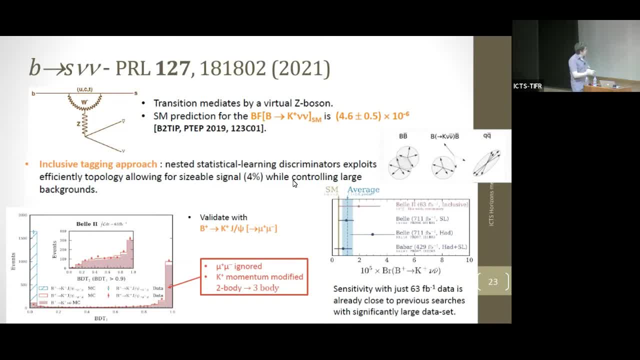 about the new physics That might be there in the charged leptons. So we've developed inclusive tagging approach which exploits differences in the shape of the events. When you compare our BB bar events in the center of mass they're produced almost at rest, So they're isotropically distributing. 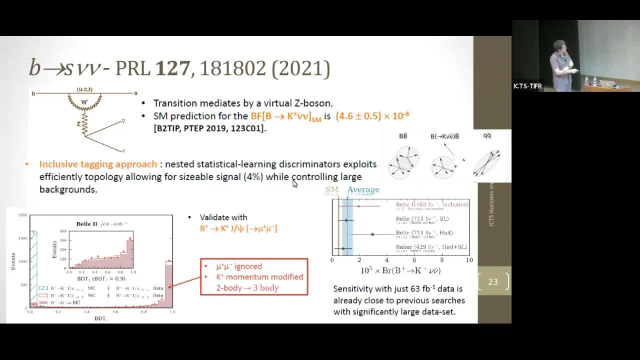 the particles over the four pi acceptance of our detector, Whereas a QQ bar event is kind of jetty back to back to one another. So you can easily distinguish- not easily, but you can distinguish between the four pi acceptance of our detector and the QQ bar event. 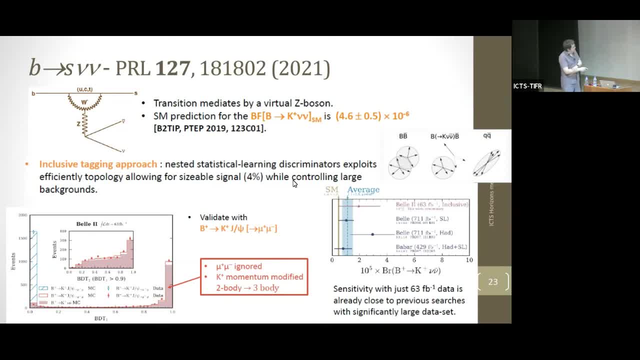 So we can easily distinguish these two types of events based on their topology. Now this K new new bar is interesting because it sort of lies between the two. You have one regularly decaying B, You just have a single track on the other side. So what we do is we train multivariate algorithms to distinguish our signal against QQ bar and then against BB bar, And we use a series of nested BDTs to do this, And we can get around a 4% efficiency for selecting these events. We also can use 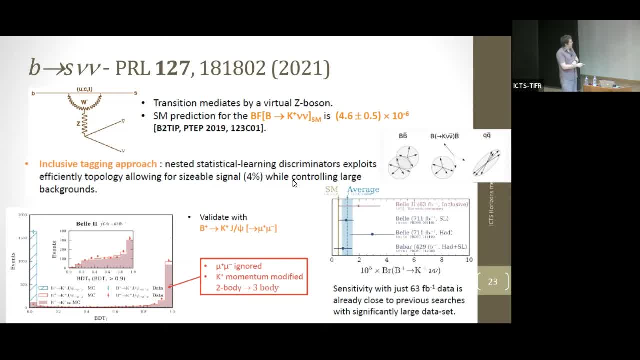 more tree level BDK processes such as BDK, JPSI, where we ignore the muons to sort of fake our signal And we even alter the kinematics so the kaons look like those coming from a three-body decay. And what we find? 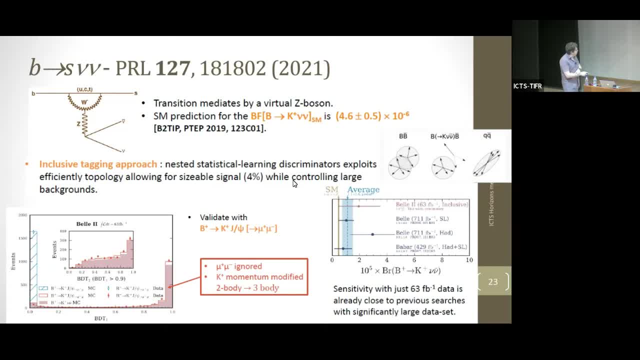 is that our data agrees well with our simulation, So that gives us confidence in the result. So, just using only 63 inverse femtobons of data, this is the purple measurement up here, which is competitive with other measurements that have been made in the past And clearly. 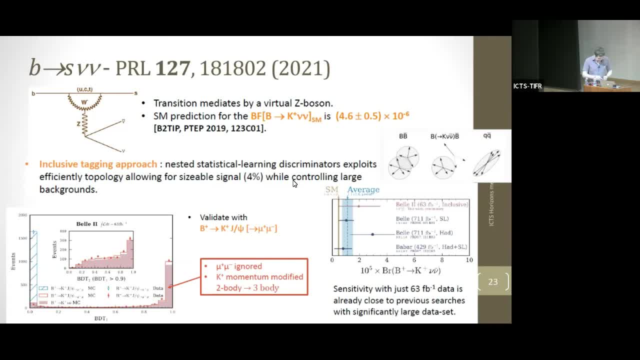 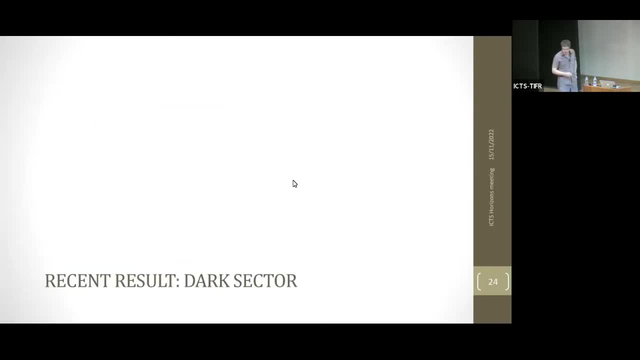 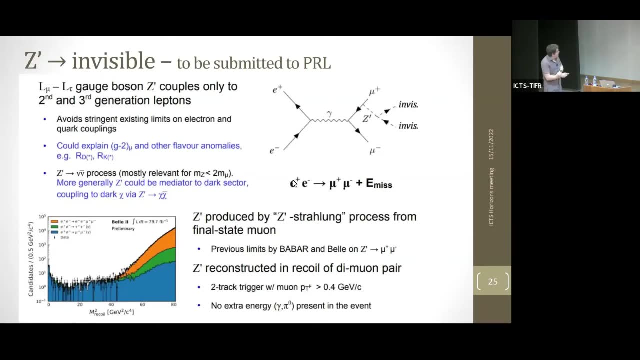 now we have five times more data. We will update this soon So we'll be able to say something about the anomalies, hopefully before too long. So my final physics topic before I conclude is just something on the dark sector. So there's a lot of interest in certain models. One here is: 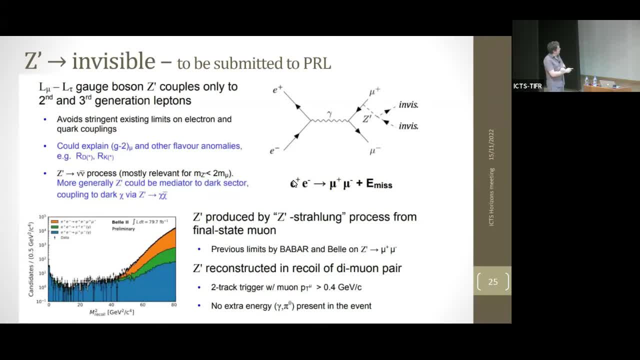 L nu minus L tau scenario. We have a new gauge boson, the z prime, which couples just to the second and third generation, So you escape all the constraints that are there from electrons and quark couplings. And this is of interest because it can explain G minus 2 and is also 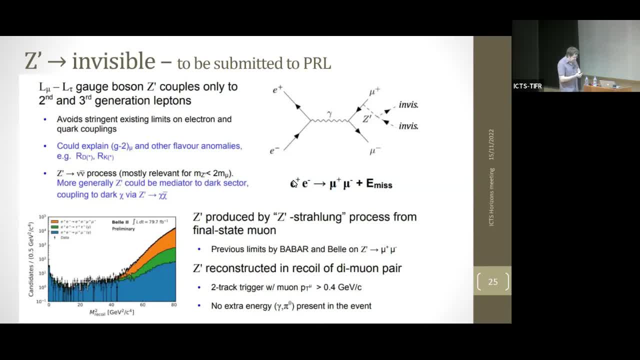 possibly related to the other anomalies that we see in the B sector. So this signature is quite clean in our environment. What we have is E plus E minus, going to mu plus B minus, And we have a z prime Strahlen process off one of the muons because it can couple to that. 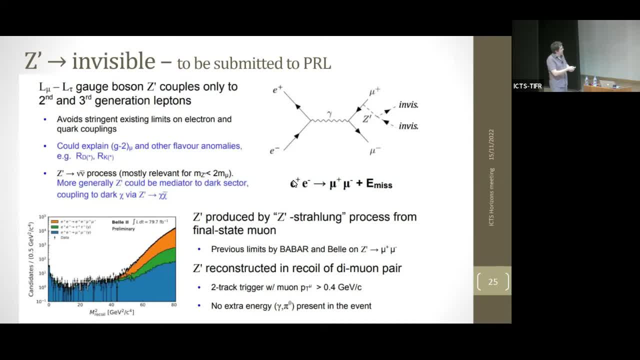 And then we're interested in particular to the z prime coupling decaying invisibly. This can happen if it goes to neutrinos, But more interestingly, it can couple to the dark sector, And then you'd have your z prime going to chi chi bar as a dark latter candidate. 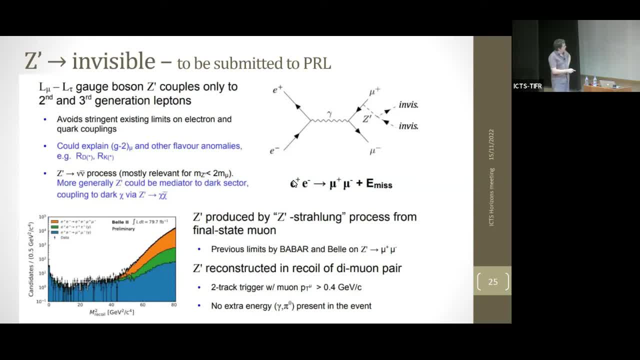 So our signature is just a pair of muons and lots of missing energy, And we can work out the recoil from our constrained kinematics. So this is the recoil mass here And we can search across this looking for a peak which would correspond to our z prime. 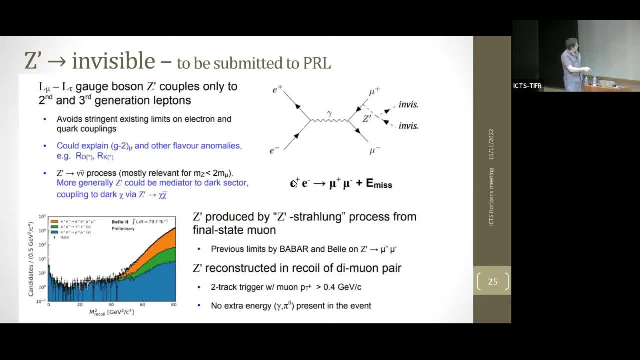 So there are various backgrounds that are more dominant at different regions of the recoil mass. You have full fermion processes and then you have radiative mu plus, mu minus and tau plus, tau minus as well, where you miss the photon. So there's been careful studies of 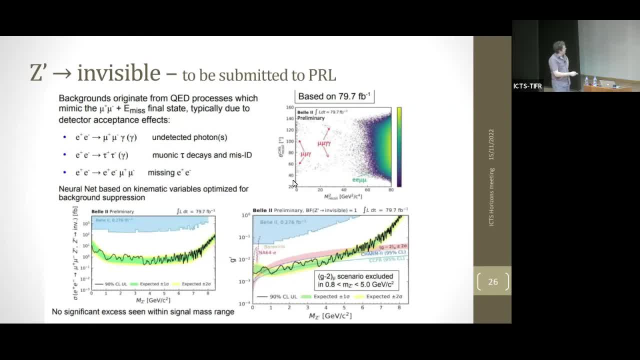 the backgrounds. There are certain gaps in the detector which we know about, and we veto those And we can turn this then into a cross-section as a function of the potential z prime mass. So this is the regular expected limit against what we see as a function. 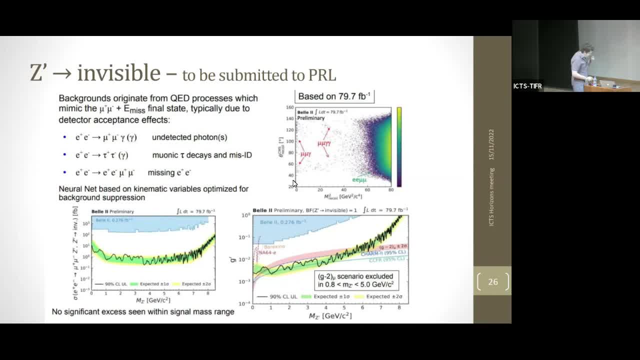 of scanning along in the mass. Unfortunately, we don't see anything. Of course you would have heard if we had, But when you recast this in terms of this L nu minus L tau model, you can compare to what you might expect the couplings to be. if it could explain the G minus 2, which is the pink. 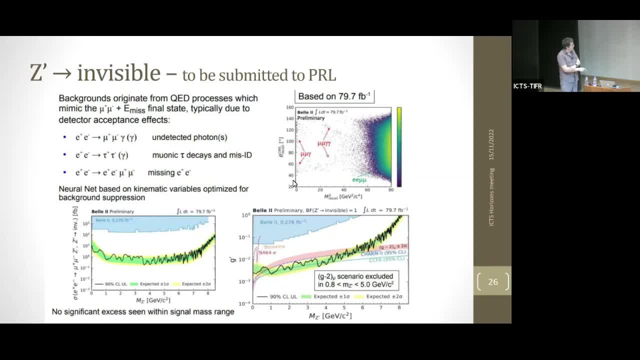 band here And, as you see, we are actually excluding a significant region of the Mz prime mass. that could explain this. with this measurement- And this again is being done with very little data, just 80 inverse femtobonds of data. So it will improve with time. So in my last few moments, 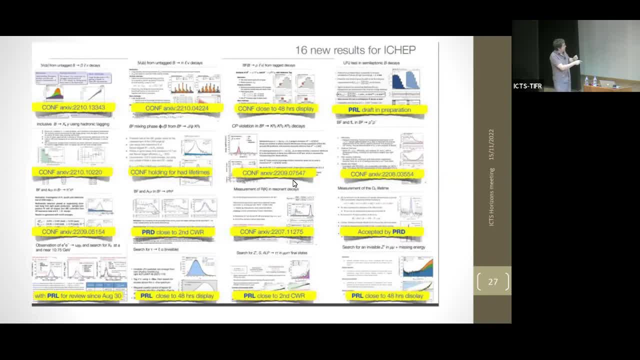 I have to address one thing. Oh no, Just to show you actually, before I get to that we have many other results. We had 16 new results for iCHEP, spanning semi-leptonics, decays, CP violation, quarkonium, tau, physics, dark sector and one more charm: lifetime. 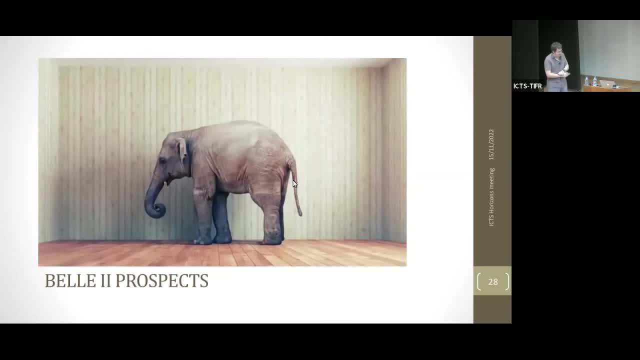 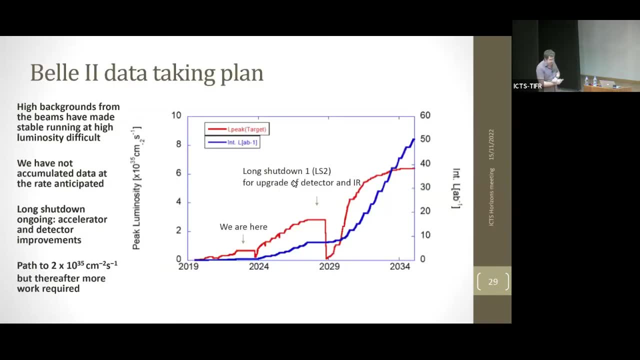 But there is a local thing we have to address. There is an elephant in the room with Bell 2 and its prospects. Those of you with a memory like an elephant will know that we have been claiming for a long time that Bell 2 would have around five inverse hasobonds of data by now. This has not happened. 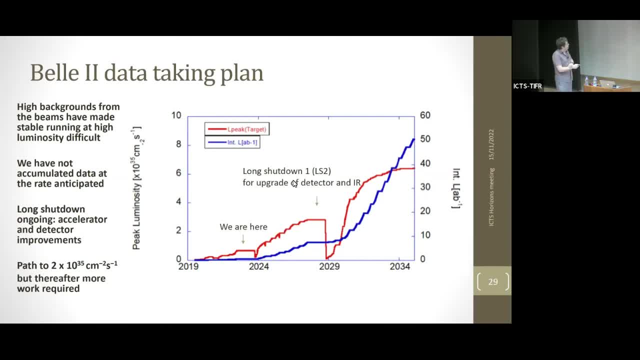 There are various reasons for this, but it's largely down to the fact that when you're trying to produce the world's largest luminosity collider, there are problems, And we've suffered greatly from backgrounds within the detector which have been so high that we've had to abort the beans. 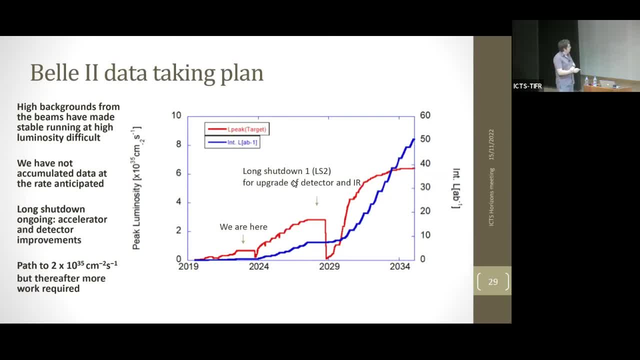 There have been lots of losses of beans very fast In the accelerator and lots of problems in injection. So we have not got to where we wanted to be And we've now had to revise our plans such that Bell 2 is running well into the middle of the next decade to possibly get 50 inverse hasobonds. 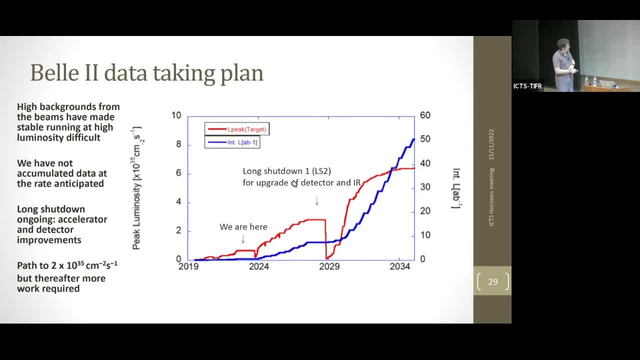 But to be clear about this, we are here at the moment We are shut down- to make improvements to the accelerator and to install our whole vertex detector, And then there is a path that we can actually enter the quite exciting 10 to the 35 inverse centimeter squared regime. 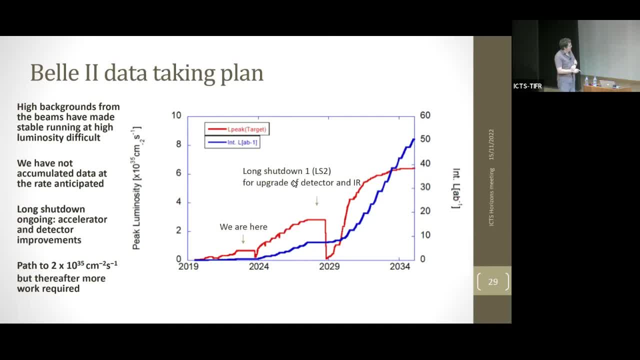 And accumulate a data set before we shut down again by around the end of 2026 or 2027, which will be multiple hasobonds, five or six inverse hasobonds probably. Then we have to do a serious upgrade of the whole detector to push up to get to the very 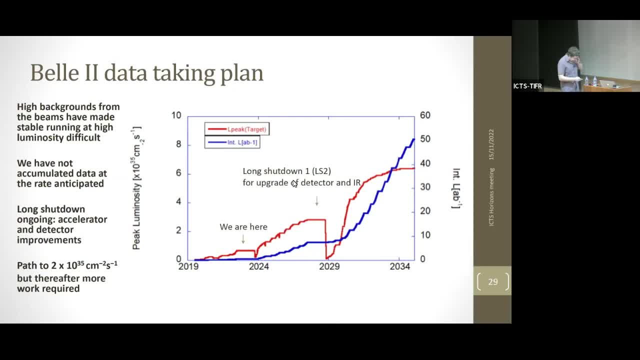 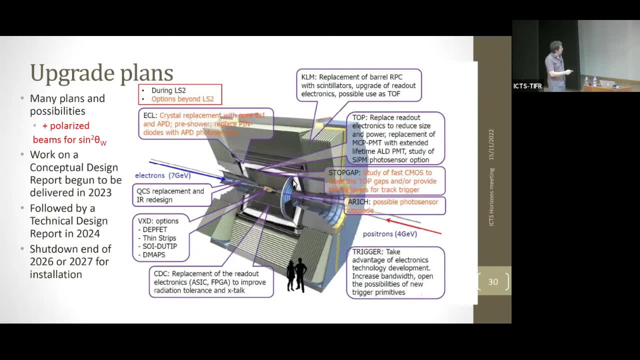 high instantaneous luminosities in the very large data sets. So people are thinking about- well, actually very actively now, thinking about upgrading Bell 2 when we are shut down for this long shutdown to improve the accelerator, And one of the key things is we 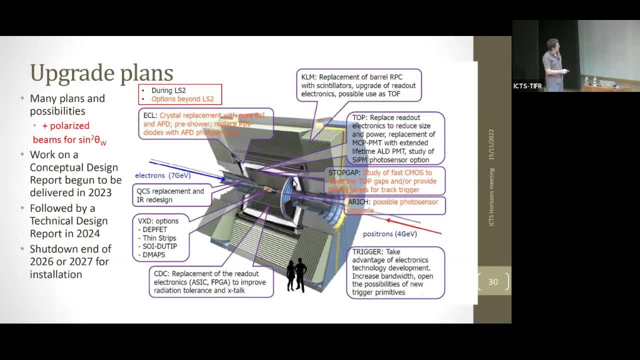 have to change the final focus, which means we essentially we have to change our silicon detector as well, And various things about the tracking and whatever will change around that And we can use this opportunity to make further upgrades. So this is ongoing process. We expect. 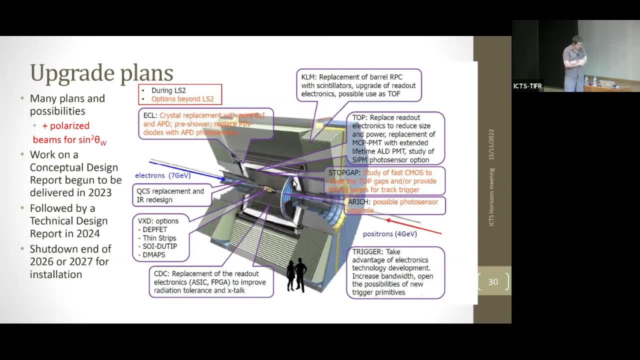 a conceptual design report this year, a technical design report next year, And we're looking to be ready to go three years after that. These are incremental upgrades, Probably the biggest of which is for the VXT. So I should conclude- I'm now 30 seconds over time. 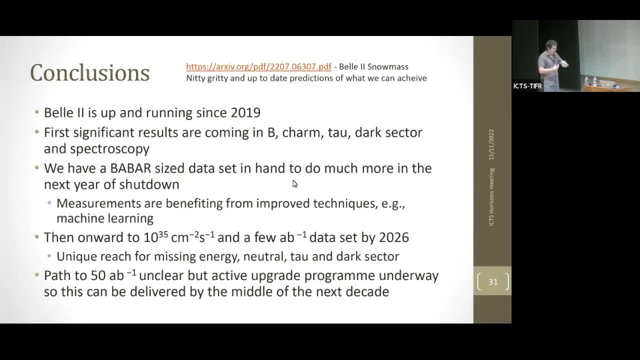 Sorry If you're interested in lists of how our precision is on these key modes over a period of time. we did this exercise last year for SNOMAS and this is the link to the report. But I just want to hopefully show you we're up and running, we're producing physics. 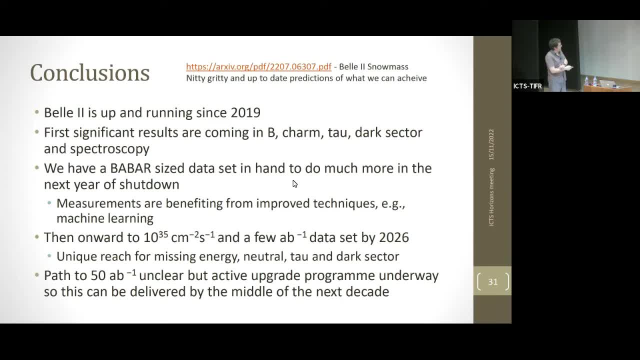 And we've now got this quite large data set, similar to what Babar had, And we're going to exploit that as best we can during this long shutdown period And we'll be getting some interesting results in the next year or so And we're benefiting from. 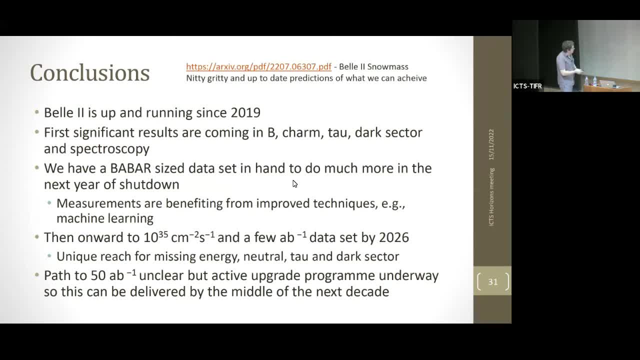 improvement techniques, particularly machine learning, But then we'll push on into this 10 to the 35 regime And we will then lead on various measurements particularly related to missing energy, neutrals, tau and dark sector And the 50 inverse Atterbarns is unclear, but we're working. 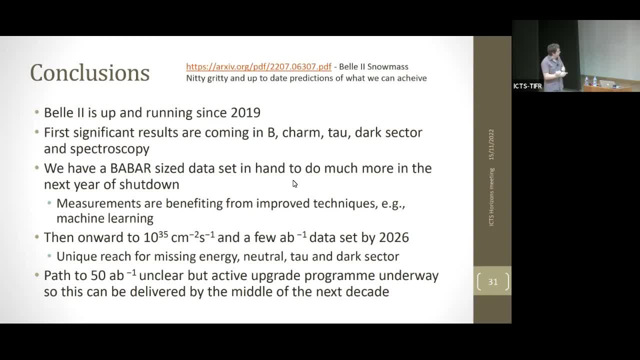 hard on this And it's a long-term program that we hope to tell you more about in the years ahead. Okay, Thank you. Thanks a lot, Jim. Very wonderful talk actually. Paulos, yeah, The Z prime in the dark matter, kind of thing that you just said. 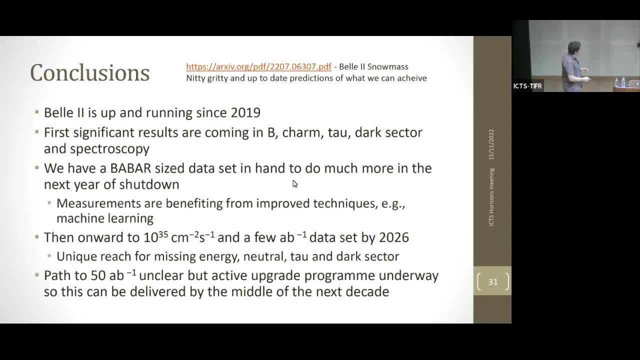 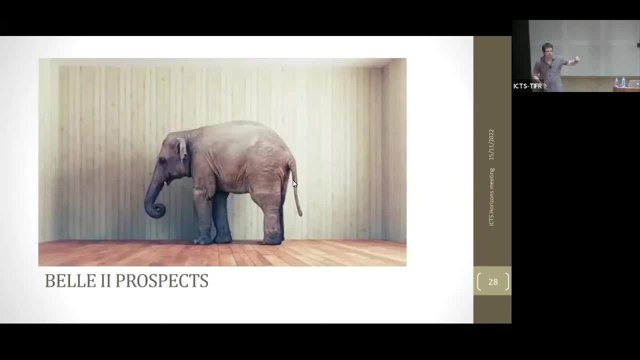 What was the mass? It's too light, for How would LHC search us? It's very light, So we've excluded in the range from just below 1 GeV up to around 5 GeV. I mean that's already a. I mean, what about the LHC Z prime kind of? 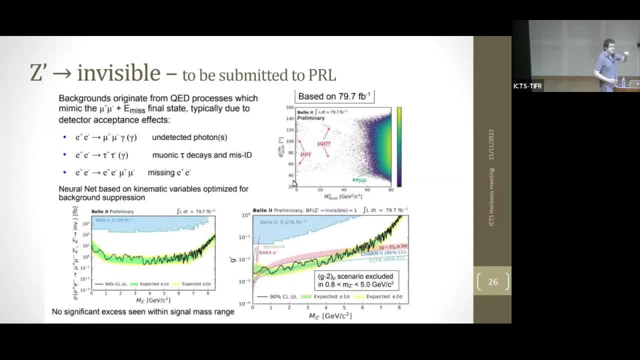 So what's key here is this: is Z prime to invisible. So if there's a coupling between the Z prime and the dark sector, that could well saturate the branching fraction. okay. So these are the first limits on a model of the Z prime. 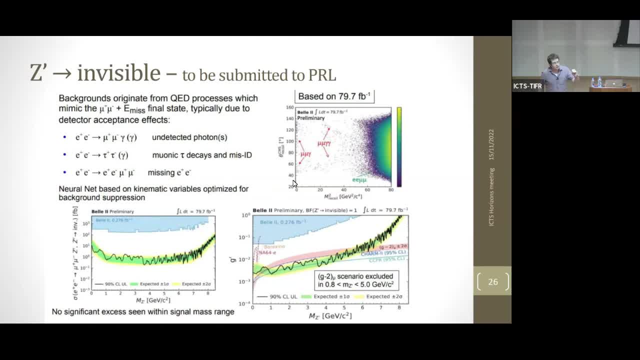 Which is decaying to dark matter. 100%. Yeah, Of course, when you look for the Z prime going to dimuons or dielectrons or something else, you'll get much more stringent limits, But there's models that predict that if 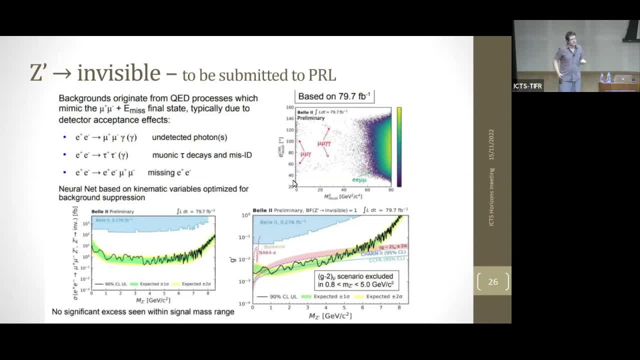 you couple to the dark sector, you will end up with this being the dominant decay mode, So you wouldn't see it there. Okay, I have two small questions. I noticed that you have 7 GeV on 4 GeV. That's a mistake. 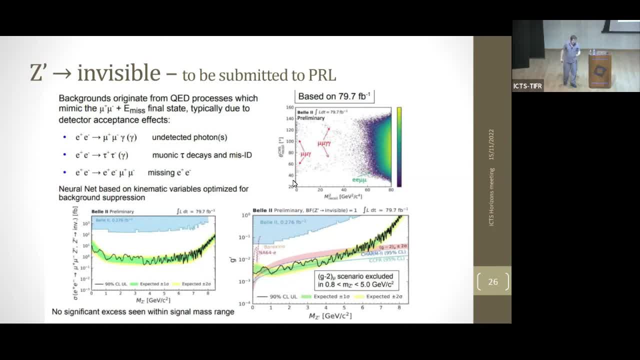 That is different from 8 on 8.. Yeah, yeah, That's the other. Why is that? Because Because I didn't check my slides carefully. That's the Bell numbers, Okay, Okay, Or is that Yeah, Or is that a typo or something? 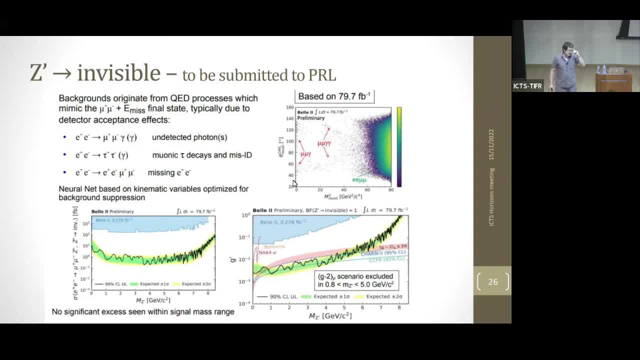 Okay, That's a typo, The. I had 8 earlier, which is the wrong way around. right, I got Anyway. Okay, The question is Keeping me honest, Vivek, Direct violation that you'd like to observe. 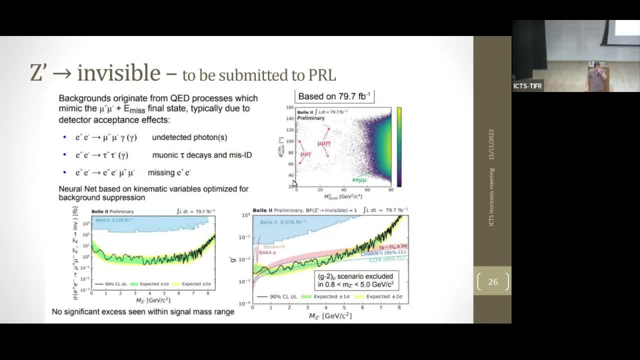 Sorry, I missed that. Direct symmetry violation. Direct T I didn't talk about today. Time-dependent CP violation. Oh, That's doing it. That's doing it as a function of the decay time. Okay, To do the T-dependence, you have to create these T-odd observables. 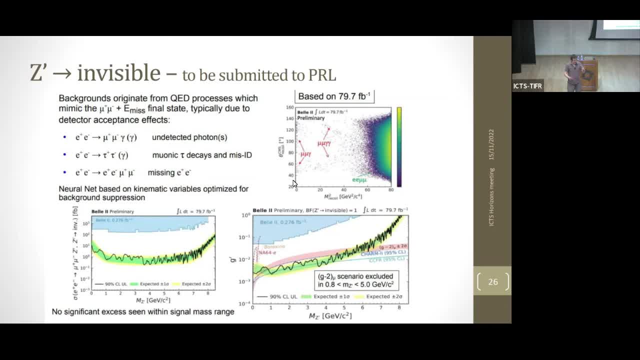 Mm-hmm. Yeah, So those are four-body final states where you create these triple products. That is things that people will do, but that's also being done elsewhere. Rohini Jim, just one quick question. Thanks for a really wonderful talk. 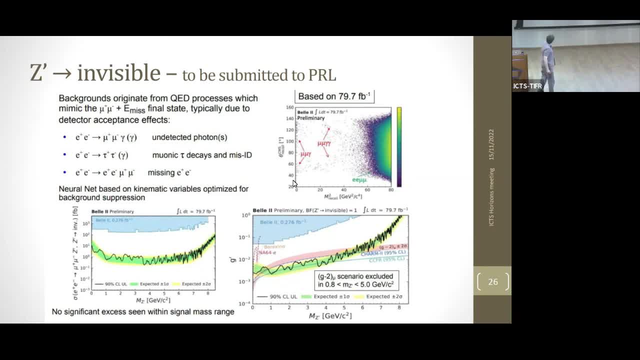 These limits that you have on Z prime, I mean these. You mean to say these regions are allowed After the, In spite of the invisible decay limits from LEP on Z prime? Yeah, I see So these are. So the only limits that come are from recasting some neutrino results. 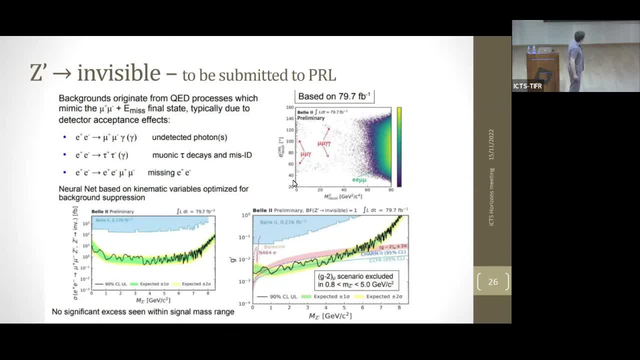 I believe from these experiments. Why does LEP doesn't have? LEP had pretty good limits on invisible branching ratio. I mean, that's how we excluded the fourth generation. This is Z prime, right, It's a Z Yeah. 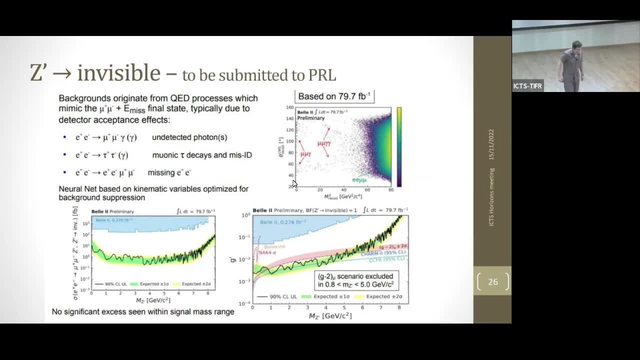 Which doesn't couple to the electrons. So we never made them at LEP. It's so very special. Well, if it exists, we never made them at LEP. so Yeah, I have one question. Yeah, Thank you. 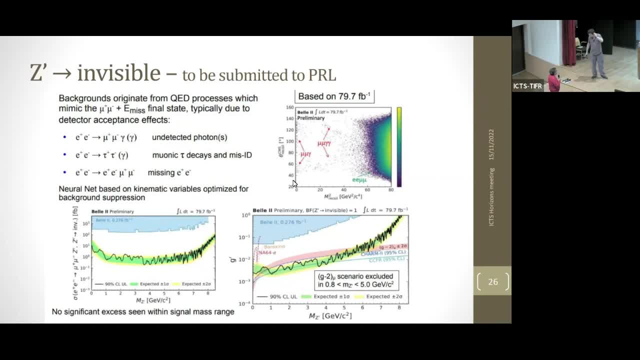 What you're going to do with charms, Manik? What are the physics measurements you're going to do with charms Charm? Yeah, with charms, We've measured the lifetimes. So, okay, as was discussed by Rukmany, LHCb has measured. 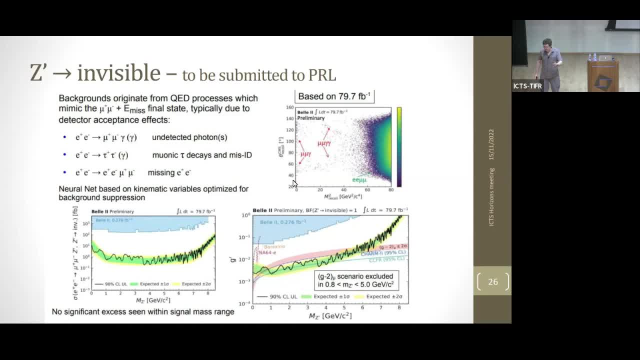 very precisely now these x and y parameters. so the mixing measurements are very hard for us to make any competitive measurement on. however, there are sort of direct cp measurements that we can make, in particular because these cps images have been seen in kk and pi pi, or particularly pi pi. 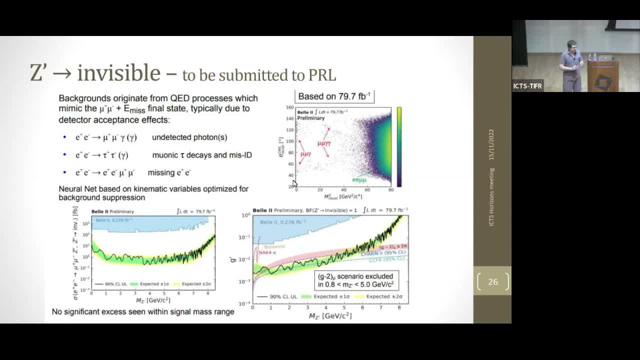 we can do pi zero, pi zero, which is cannot be done at lhcb and with a very large data set, we should have a precision which is able to probe the region that's being seen by lhcb. so there are other modes with neutrals, which we can do really well. however, you know classic mixing and time-dependent. 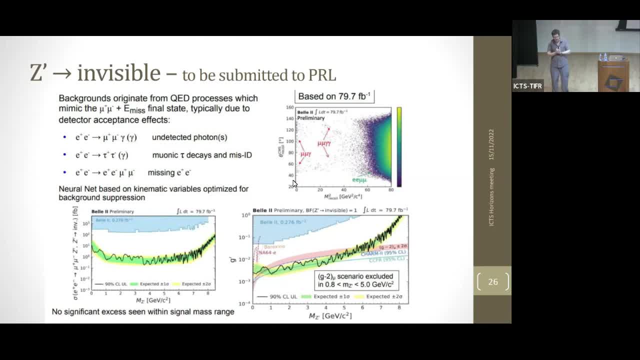 measurements are really quite tough for us compared with the great progress that lhcb has made over the years. thanks a lot, you have a good. so at the present, no, we want to accumulate as much data as we possibly can with the epsilon for us, so there are some plans for potentially doing scans to do quarkonium in that region. 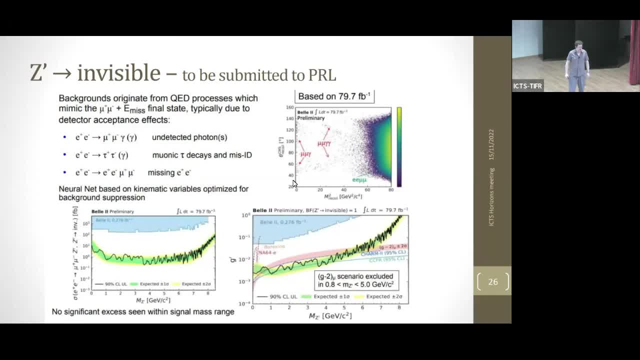 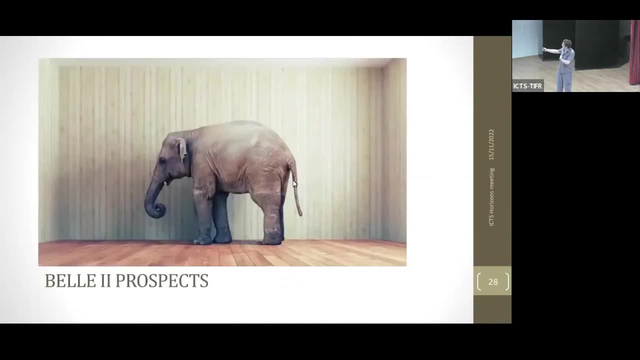 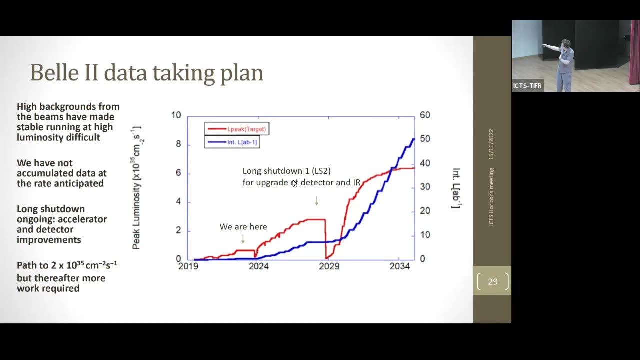 but at the moment there is there is no plan to take a significant amount of time to do that away from the 4S program. Once we're in this regime, yeah, we would certainly consider taking time away from the 4S, But for now, given anomalies, given all these things, that's the focus. 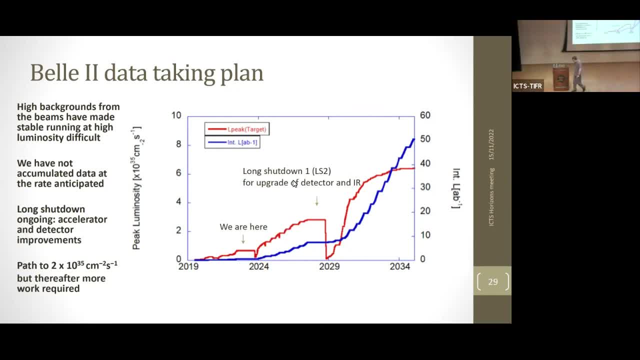 Okay, one last question, Manoraji James, in continuation with the Z prime thing in the LEP, there is a data missing momentum, along with the photons. that can rule out the Z primes to some extent. Is it looking for So you're talking about? 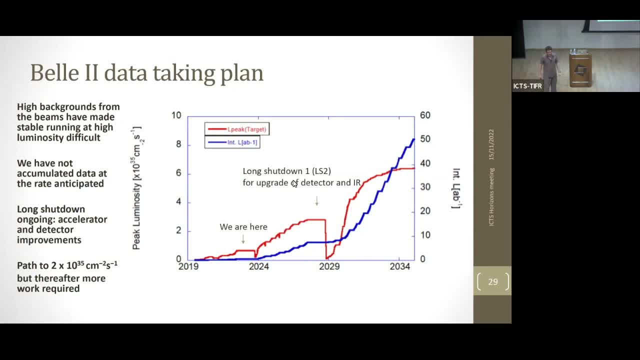 LEP data. LEP data: LEP data means missing momentum, along with the monophoton type of thing. Monophoton, again, because you didn't produce the Z prime, because what was it? The Z prime gives you the missing momentum. 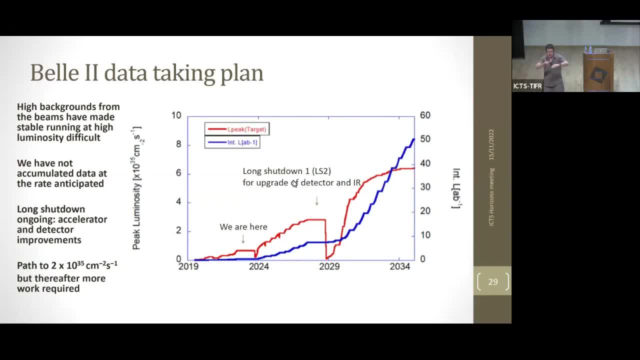 Haha, but this is Rohini's question. Your Z prime is coupling to the leptons, right. So you'd have to have the Z prime coming from a mu plus, mu minus or a tau pair. this Z prime Strahlen process, It's the production. 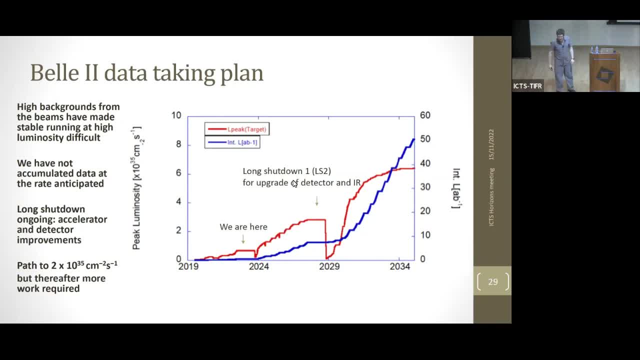 L mu minus L tau, Mix with: yeah Right, Pius, Yeah, Just a quick question: Have you updated the bounds on axion-like particles similar to the Z prime? So we haven't updated that. Where did that come from? It's very disorientating, Sorry.